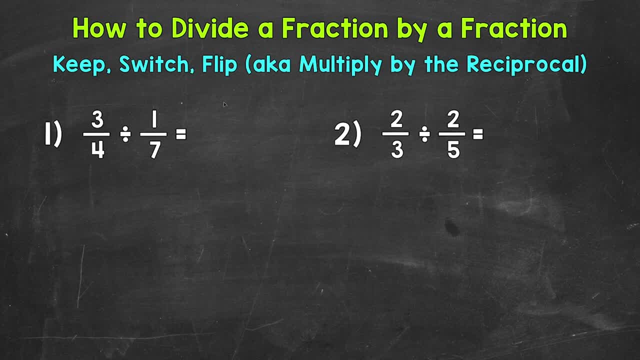 This actually makes the process simpler. Now, how and why this works, that's something I'll cover later in this video. Let's jump into number one, where we have three-fourths divided by one-seventh. So we are seeing how many one-sevenths we can make out of three-fourths, or how many one-sevenths 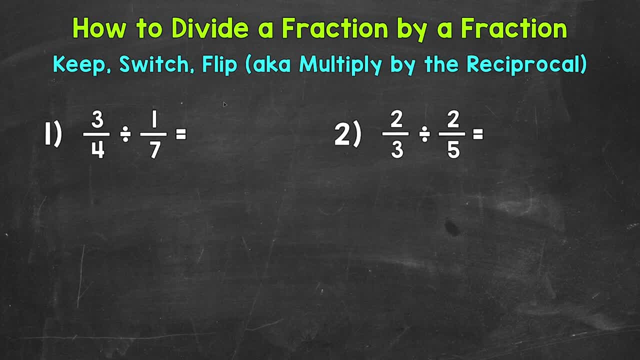 are in three-fourths, so to speak. So let's start by rewriting this problem using the multiplication method. We're going to take a look at how to divide fractions by keeping switch flip. So we always keep the first fraction or number. So we keep three-fourths. 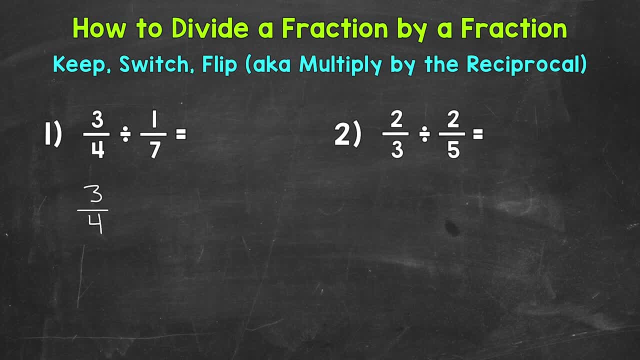 as is, We switch to the opposite or inverse of division, which is multiplication. And since we switch to the opposite or inverse of division, we're going to flip the second fraction. So the seven is going to be our numerator and the one is going to be our denominator. So we're going to 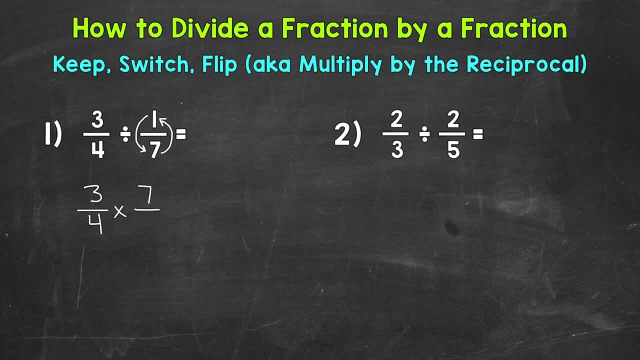 end up with seven over one. Once we get to this point, it's a multiplying fractions problem, So we can multiply straight across: Three times seven is twenty-one, and then four times one is four, And we end up with twenty-one-fourths. Now that's an improper fraction, so we do not want to leave it. 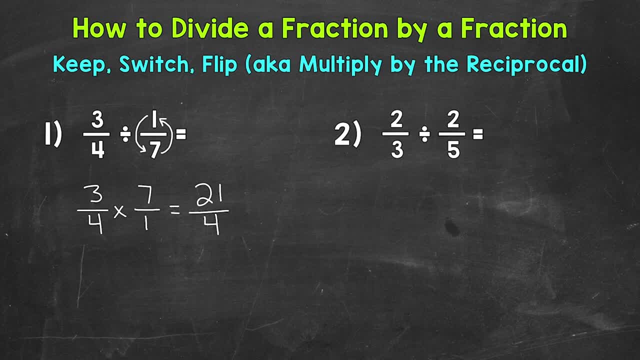 We need to divide our numerator of twenty-one-fourths by one-sevenths. So we're going to multiply twenty-one by four. How many whole groups of four are in twenty-one? Well, five, That gets us to twenty. So five whole groups of four, That's our whole number of the mixed number here. Now that 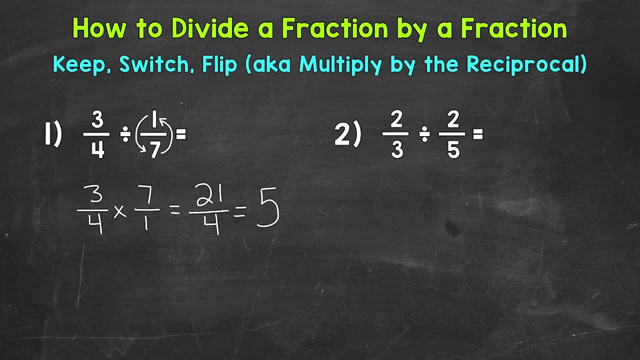 doesn't hit twenty-one exactly, We have a remainder of one. So that's our numerator in our fractional part of the mixed number And we keep our denominator of four the same. Always. look to see if you can simplify the fractional part of the mixed number. So we're going to keep our denominator. 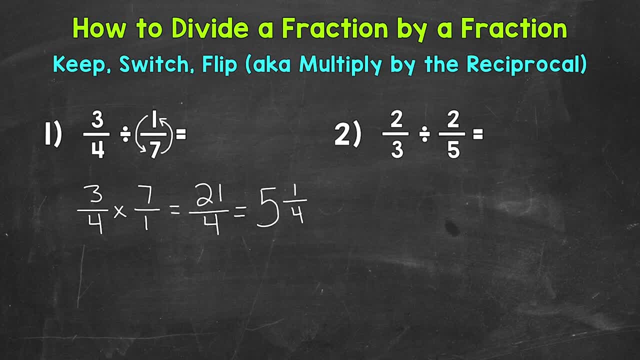 of a mixed number. One-fourth is in simplest form. So we are done. Five and one-fourth is our answer for number one. So three-fourths divided by one-seventh equals five and one-fourth. Let's move on to number two, where we have two-thirds divided by two-fifths. Keep switch flip, So keep two-thirds. 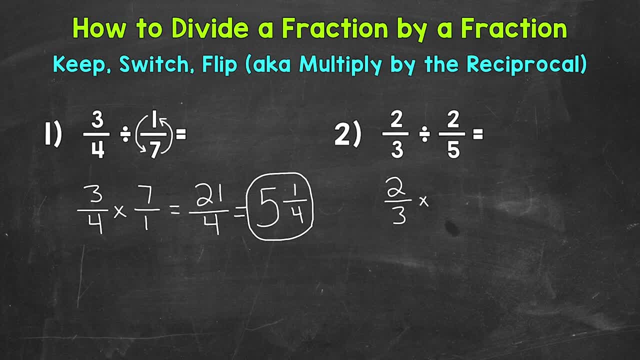 a multiplication and then flip that second fraction, So five over two, And now we can multiply straight across. Two times five is ten. Three times two is six, So we get ten-sixths. So that's an improper fraction. We need to convert to a mixed number. So ten divided by six, How many? 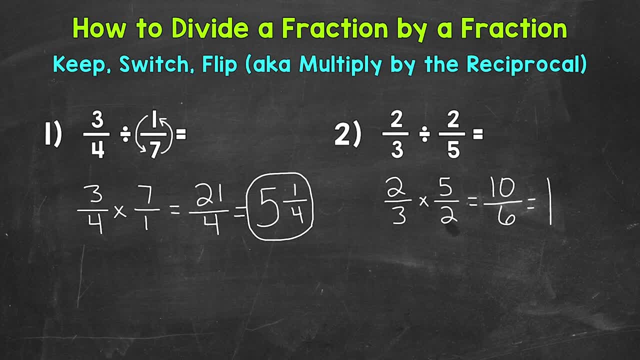 whole groups of six out of ten. Well, one, And we get a remainder of four. Keep our denominator of six the same. We can simplify four-sixths. We have a common factor of two. So let's divide each of these by two here, And we get. 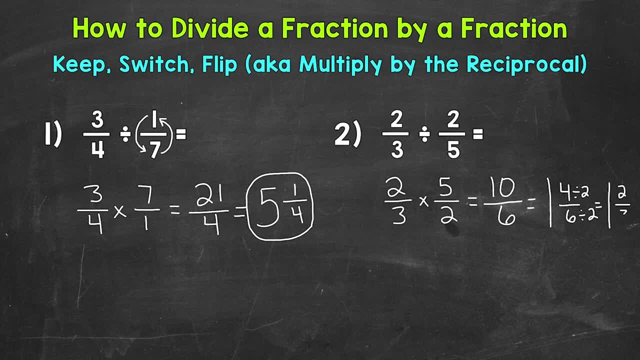 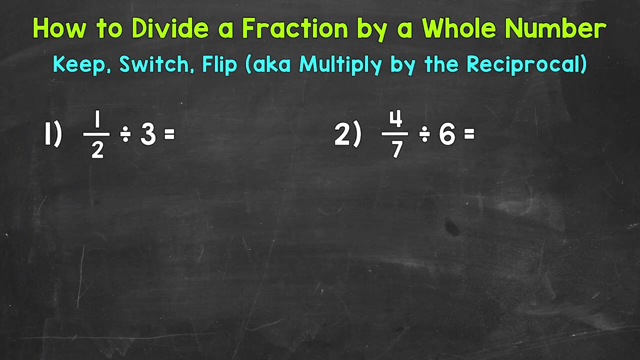 one and two-thirds. So our answer for number two is one and two-thirds. Two-thirds divided by two-fifths equals one and two-thirds. There's how to divide a fraction by a fraction. Let's move on to dividing a fraction by a whole number. Now we will take a look at dividing a. 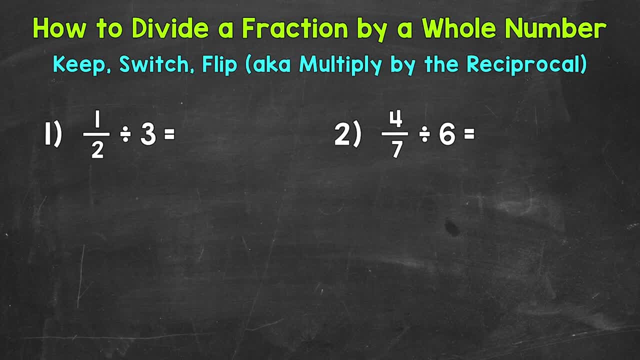 fraction by a whole number. Let's jump into number one, where we have one-half divided by three. So we are taking one-half and dividing it into three equal groups or parts. Let's rewrite the problem using keep switch flip in order to solve this. So always keep the first fraction, or 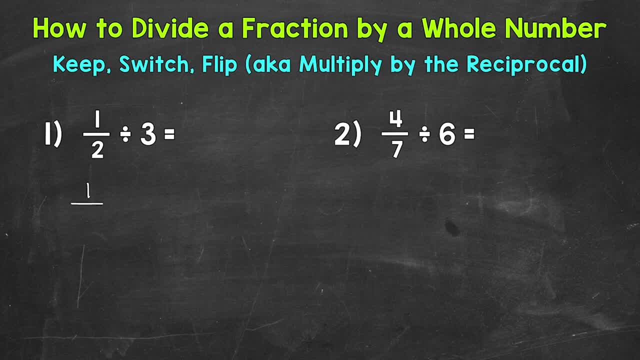 number. So let's rewrite the problem. So one-half we are going to keep. Then we switch to the opposite or inverse of division, which is multiplication. And since we switched to multiplication, we need to flip the second number or fraction. In the case of number one, we have a 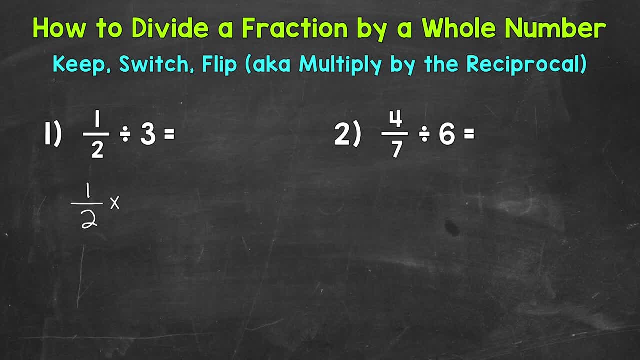 whole three here. So how do we flip this? Well, let's put that whole number over one. That way we have a numerator and a denominator That does not change the value of the problem, That still has a value of three. So now we can flip, So the one is going to go up to the top and be our numerator. 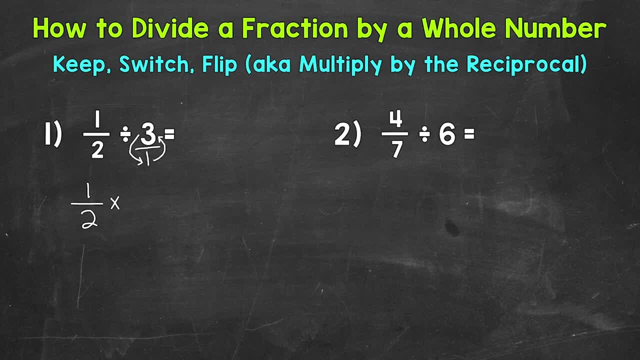 and the three is going to be the denominator. So we flipped that second number One-third. Once we get to this point we have a multiplying fractions problem. So we can multiply straight across: One times one is one and two times three is six. So one-sixth is our final answer. 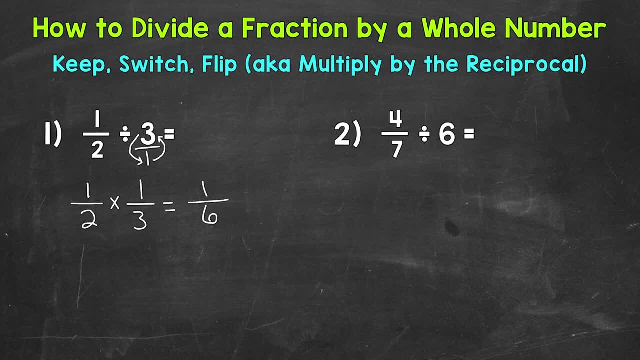 Always check to see if you can simplify. One-sixth is in simplest form. So we are done. One-half divided by three equals one-sixth. Let's move on to number two, where we have four-sevenths divided by six. Keep, switch flip. So let's rewrite the problem. 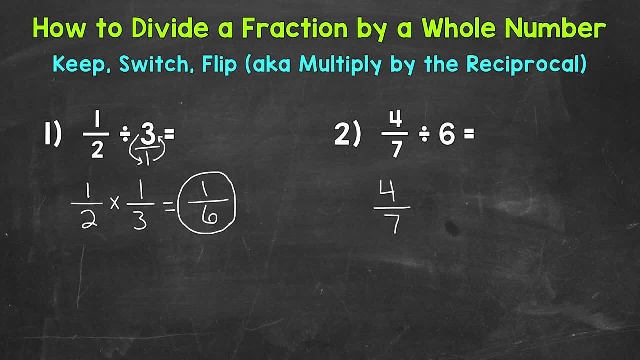 Keep four-sevenths, switch to multiplication. and then we need to flip, So we can write that six in fractional form. and now we can flip. So the one is now our numerator and the six is now our denominator. We can multiply straight across. Four times one is four. Seven times six is forty-two. 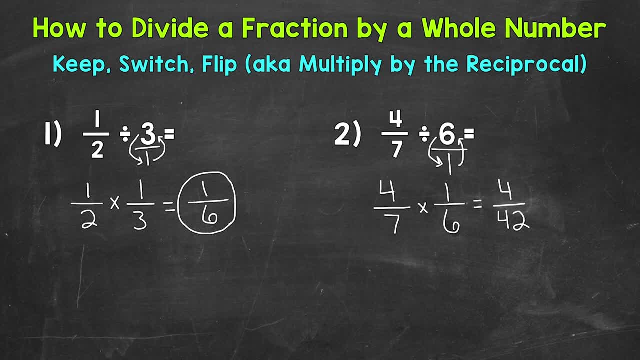 So we get four over forty-two, which can be simplified. Four and forty-two have a greatest common factor of two, So let's divide each of these by two and we get two over twenty-one. for our final simplified answer, Let's move on to dividing a whole number by a fraction. 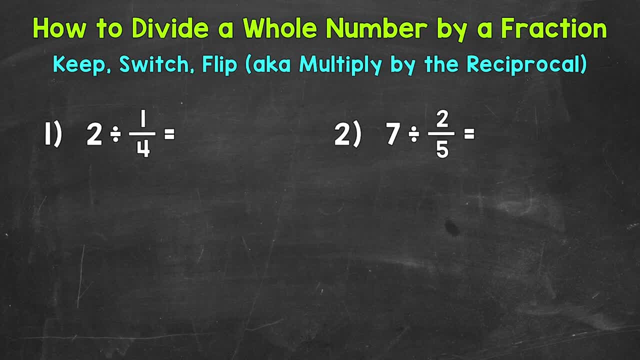 Now we will take a look at dividing a whole number by a fraction. Let's jump into number one, where we have two divided by one-fourth. Now we can think of this as how many one-fourths are in two, or how many one-fourths can we make out of two. 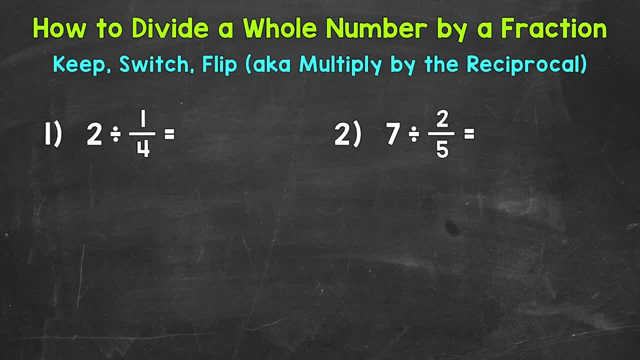 e $2234, and $1079, and a supplement of two. The question is what people can make out of two. We are dividing 2 by 1. fourth, Let's rewrite our problem using keep switch flip, also known as multiplying by the reciprocal. 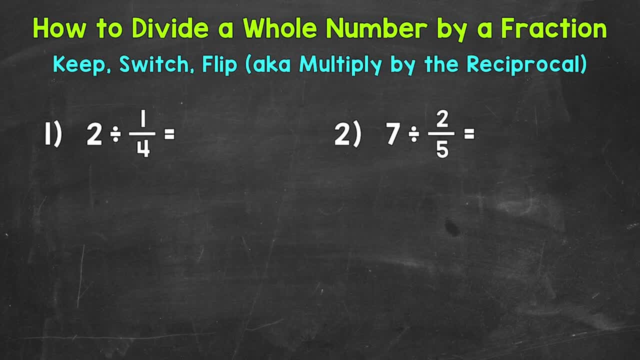 So we start with keep. We always keep the first number or fraction. In the case of number 1, we have a whole 2. So we need to keep that as 2.. But we're going to rewrite it as a fraction. 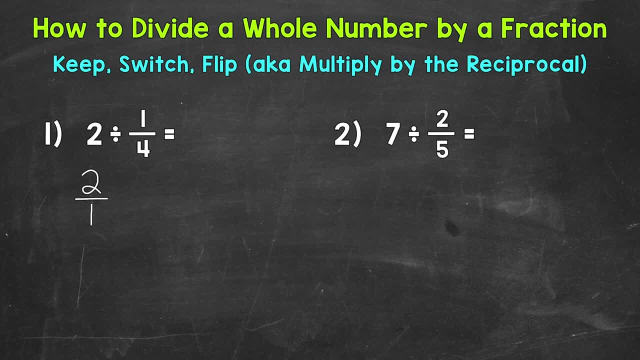 Whenever you rewrite a whole number and put it in fractional form, all you need to do is put it over 1.. Now the purpose of this: we want to have a numerator and a denominator, So we kept the value of 2 there. 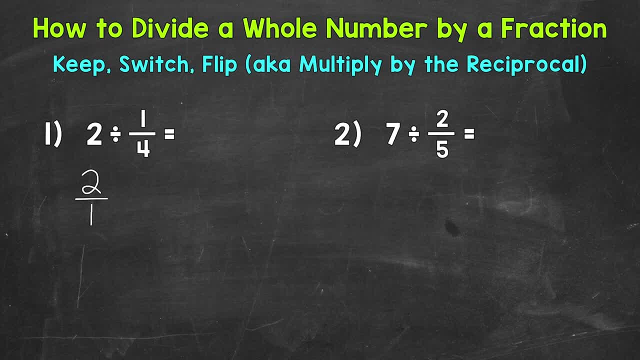 We just put it in fractional form. Then we switch from division to multiplication And since we switched to the inverse or opposite of division, we're going to need to flip The second number or fraction. In the case of number 1, here we have a fraction. 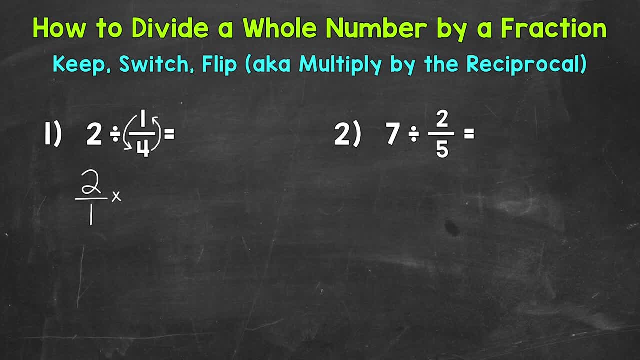 So the denominator is now going to be the numerator And the numerator is now going to be the denominator. So we have 4 over 1.. Once we get to this point, we have a multiplying fractions problem, Which we just multiply straight across when we multiply fractions. 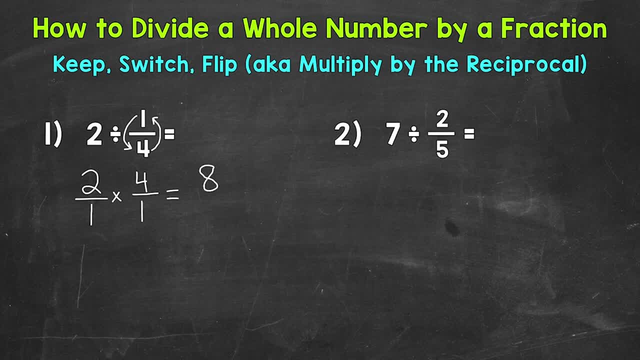 So 2 times 4 is 8. And 1 times 1 is 1.. So we get to the answer of 8 over 1, which is an improper fraction. So we do not want to leave it like that. This is going to be 8.. 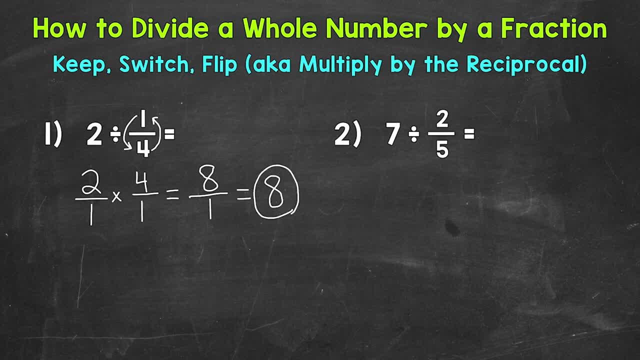 Our final answer is 8.. 2 divided by 1 fourth equals 8.. Let's move on to number 2. Where we have 7 divided by 2 fifths. So we are finding out how many 2 fifths are in 7,, so to speak. 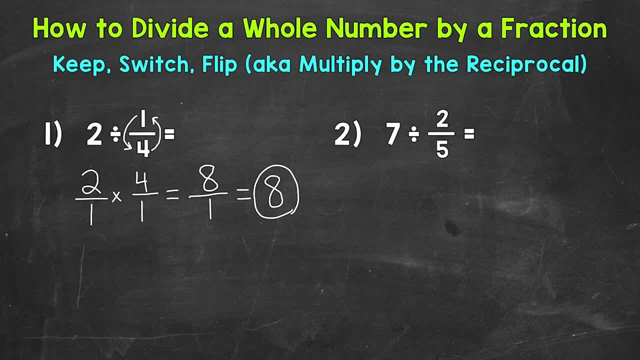 So we are finding out how many 2 fifths are in 7,, so to speak. So we are finding out how many 2 fifths are in 7,, so to speak. So keep switch flip. We will keep our 7, but put it in fractional form by putting it over 1.. 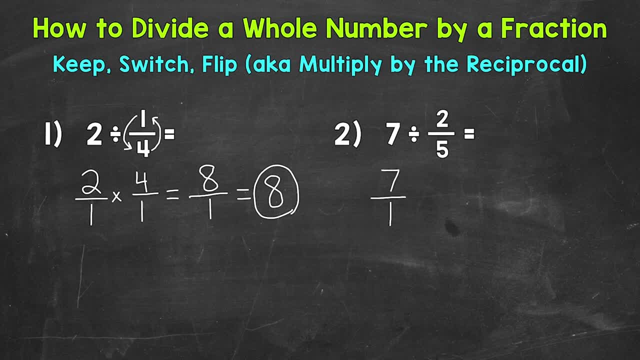 So keep, switch, flip. We will keep our 7, but put it in fractional form by putting it over: 1. Switch to multiplication And then flip our second number or fraction, And then switch to multiplication And then flip our second number or fraction. 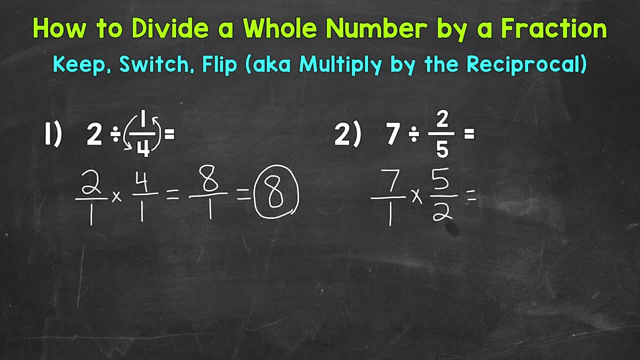 Now we can multiply straight across: 7 times 5 is 35. And 1 times 2 equals 2.. And 1 times 2 equals 2.. So our answer is 35. over 2.. Now we don't want to leave it improper. We want to convert this to a mixed number, So we do. 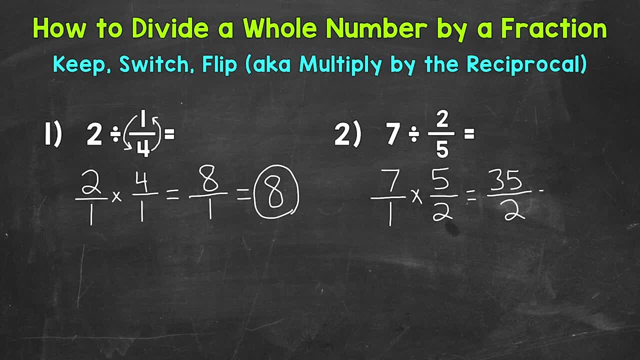 35 divided by 2.. How many whole groups of 2 are in 35?? Well, 17.. So that's our whole number of our mixed number. Now, we didn't hit 35 exactly. We had a remainder of 1.. So that's our numerator. 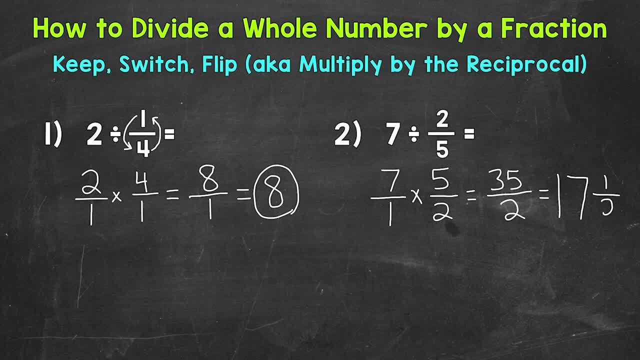 of the fractional part, And then we keep our denominator of 2 the same. So 17 and a half. Always, look to see if you can simplify the fractional part. One half is in simplest form. So we are done. Our final answer: 17 and a half. So there's how to divide a whole number by a. 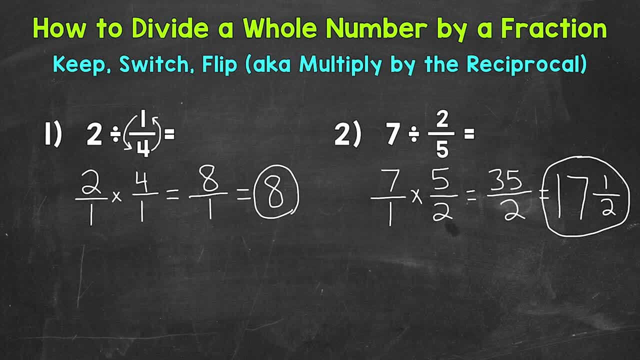 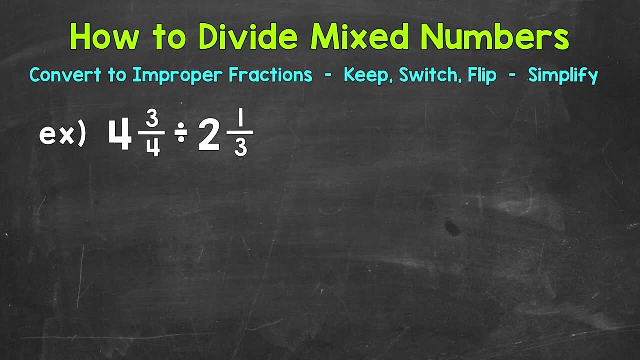 fraction. Let's move on to dividing a mixed number by a mixed number. Now we will take a look at dividing a whole number by a fraction. So we're going to take a look at dividing a whole number, a mixed number, by a mixed number. Let's jump into our example, where we have 4 and 3 fourths. 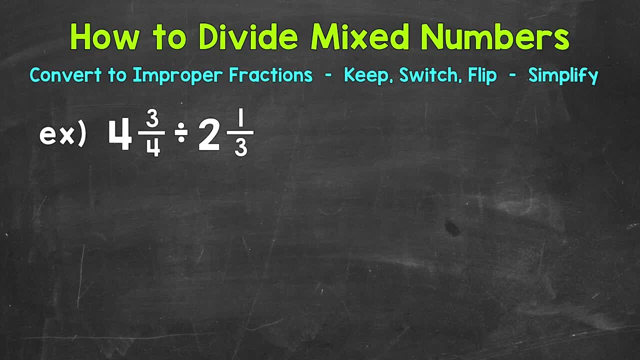 divided by 2 and 1. third. Now, the first thing that we want to do is to convert these mixed numbers to improper fractions. That way we just have a numerator and a denominator. Let's start with 4 and 3, fourths, And we start at the bottom and work our way to the top. So we 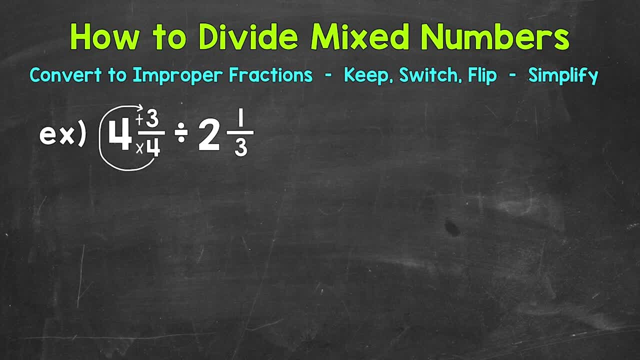 multiply, then add. So we do 4 times 4.. So the denominator times the whole number 4 times 4 is 16.. Then we add the numerator 16 plus 3 is 19.. So 19 is the numerator of our improper fraction. 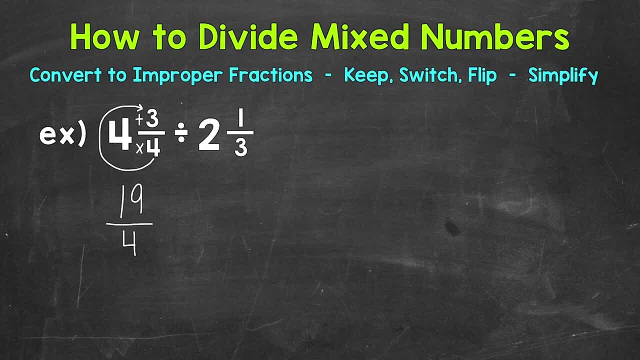 We keep our denominator of 4 the same, Then we can bring our division sign down and convert our second mixed number. So again, we multiply, then add. So 3 times: 2 is 6 plus 1 is 7.. That's our 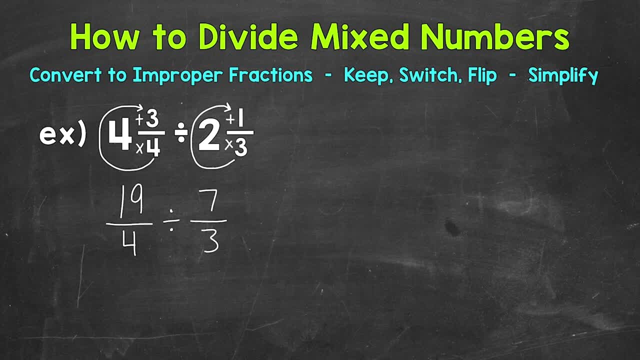 numerator And then keep the denominator of 3 the same. So 7 thirds, 19 fourths is equivalent to 4 and 3 fourths, And then 7 thirds is equivalent to 2 and 1 third. So we're not changing the value of. 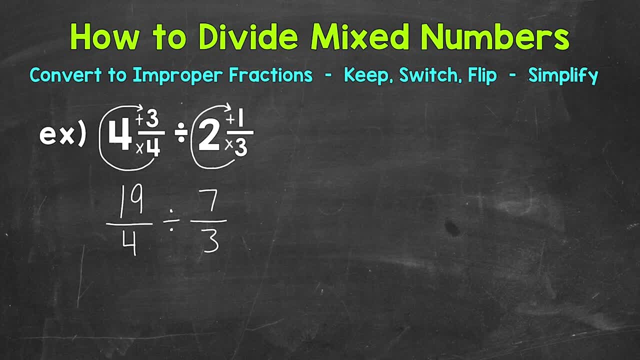 the problem at all when we convert to 4 and 3 fourths. So we're not changing the value of the problem at all. when we convert to improper fractions, Mixed numbers and improper fractions are equivalent, They're just in different forms. Now again we're converting to improper fractions. 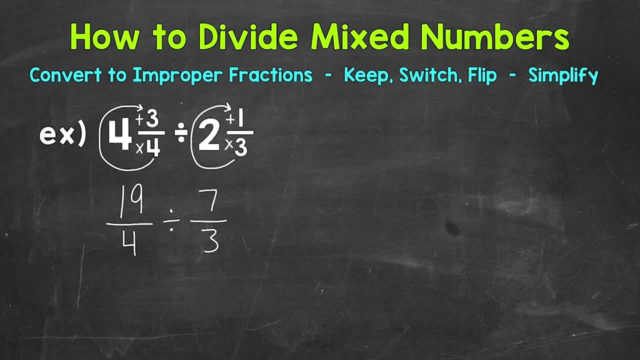 So we just have a numerator and a denominator And then we can go through our steps for dividing these fractions, Which we're going to use keep switch flip, Also known as keep change flip. So no matter how you think of it, they mean the same thing. I know there's different words out there. 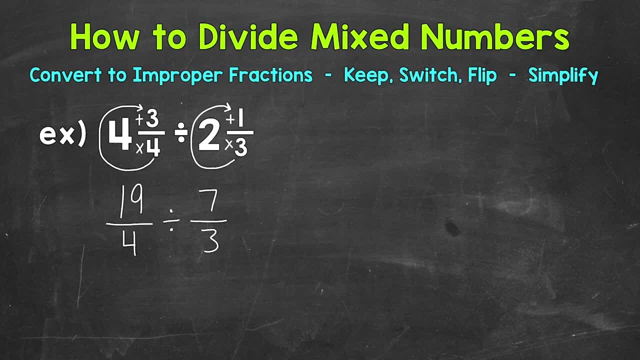 for these steps, But in the end they all mean the same thing. So let's keep our first fraction here, Our first improper fraction, So 19 fourths. Then we switch or change our division to multiplication, And then we flip our second fraction, Our second improper fraction here, So the denominator becomes: 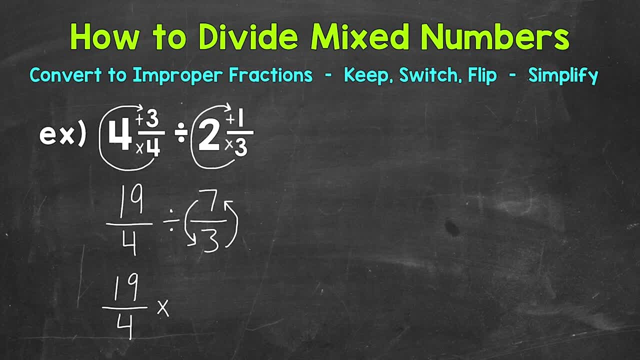 the numerator, And the numerator becomes the denominator. This is called the reciprocal. So we have 3 sevenths. Once we get to this point we can multiply straight across. So numerator times numerator And then denominator times denominator. Let's do the numerators first, So 19 times 3. That gives us 57. And then we have 4 times 7. Which is 28.. 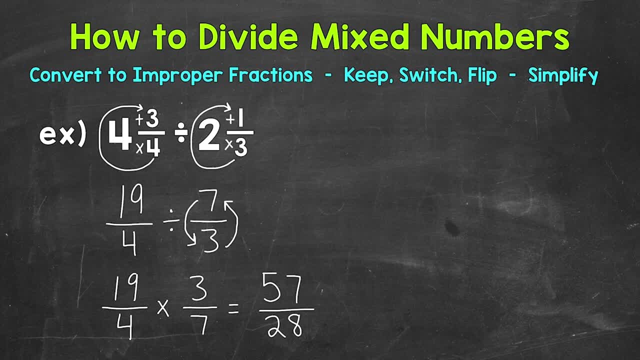 Now that's our answer as an improper fraction. So we're going to go through our steps for dividing our fraction. We're going to convert it to a mixed number, So we need to do our numerator 57 divided by our denominator 28.. Now we can do this using mental math, Or we can write everything out. 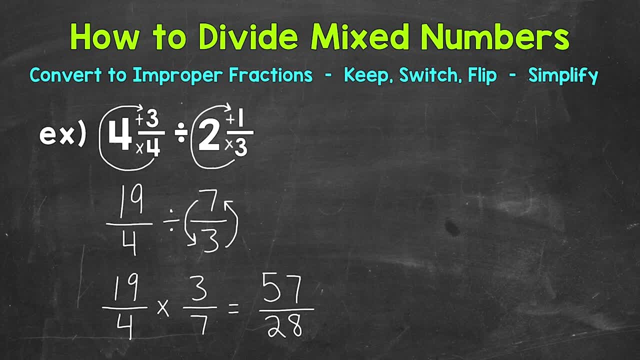 Some problems are going to be a little simpler And we're going to be able to use mental math And in some situations we'll have to write out the problem. I'll go through both here so you can see what that looks like. Let's use mental math here first. So how many whole groups of 28? 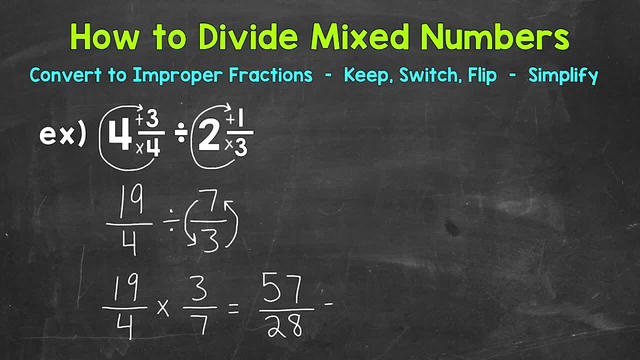 out of 28?? Let's go through both here. So we're going to use mental math here first. So how many whole groups of 28 out of 57?? Well, if you're able to think about that, it's going to be two. 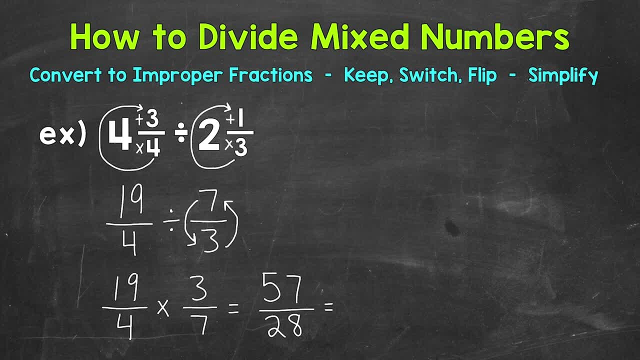 whole groups of 28. Because that gets us to 56. So two whole groups of 28.. Now we do not hit 57 exactly. We have something left over, A remainder. So the difference between 57 and 56 is 1. So we 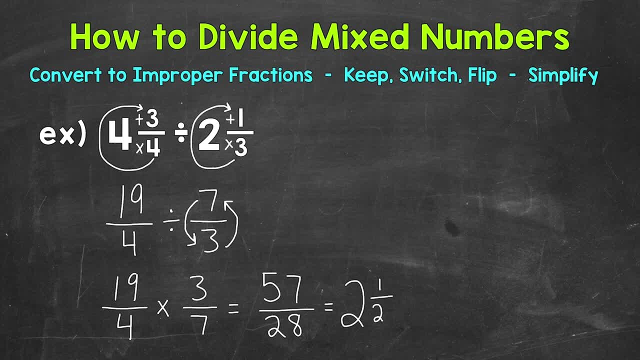 have a remainder of 1. And we keep our denominator of 28 the same. Let me write this down So we have that out as well. so we have 57 divided by 28, so we need to think how many whole groups of 28 out. 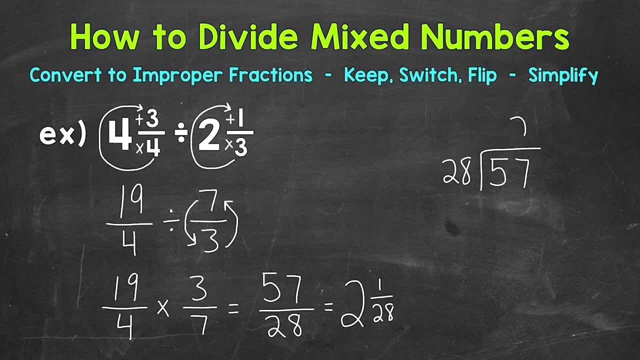 of 57. well, we said that's 2. that gets us to 56. so 2 2 times 28 is 56. so we get a remainder of 1. this 2 is going to be the whole number, part of our mixed number, 2: whole 28s out of 57. 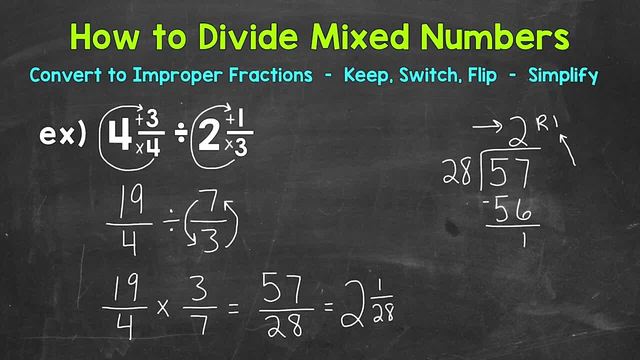 and then this 1. the remainder is going to be the numerator and then we keep our denominator of 28 the same. once we get to our mixed number, we can check to see if we can simplify the fractional part. 128 is in simplest form. the only common factor between 1 and 28 is 1. 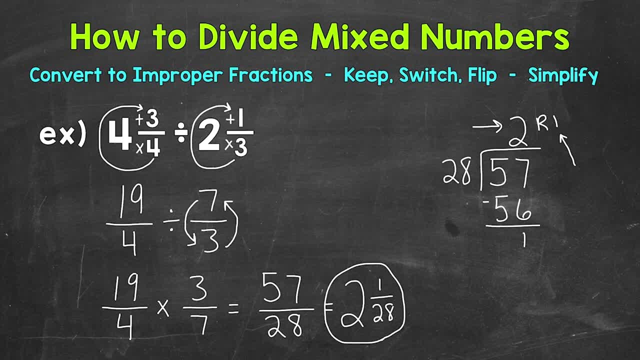 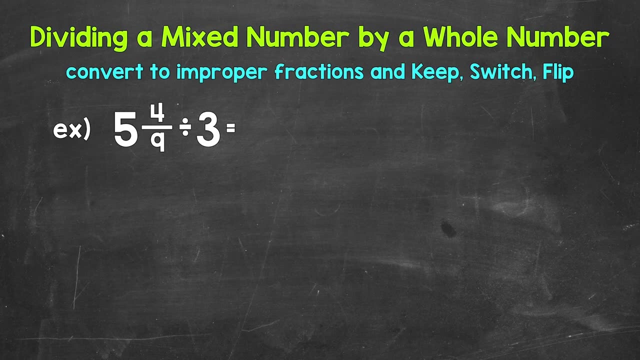 so you, We are done 2 and 1, 28th. So there's how to divide a mixed number by a mixed number. Let's move on to dividing a mixed number by a whole number. Now let's take a look at dividing a mixed number by a whole number. 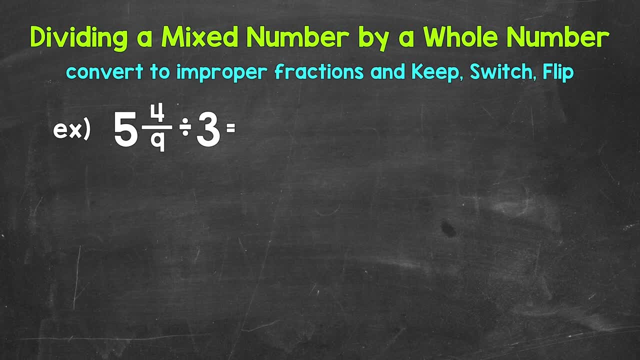 Let's jump into our example where we have 5 and 4 9ths divided by 3.. Now the first thing that we need to do is rewrite everything in fractional form. So we're going to convert everything to improper fractions. That way we just have numerators and denominators. 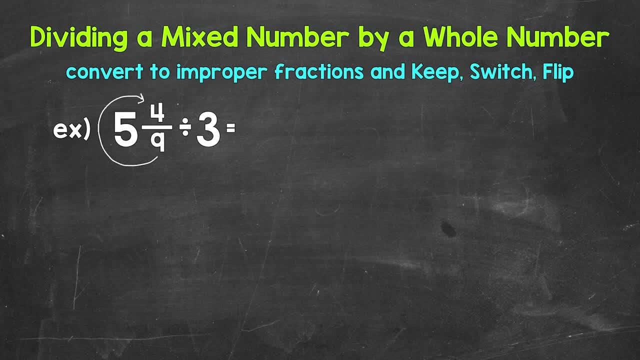 So we can convert 5 and 4 9ths to an improper fraction. first We start at the bottom and multiply and then add. So take the denominator and multiply it by the whole number, So 9 times 5. That gives us 45.. 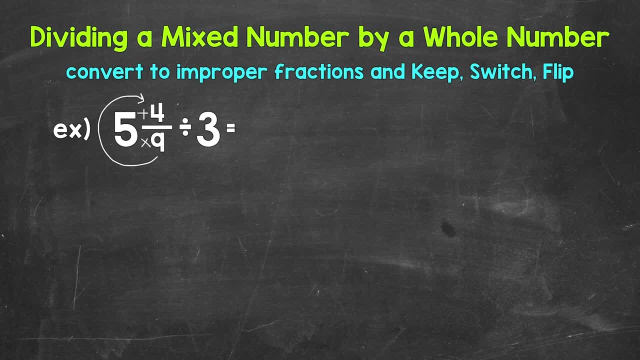 And then we add the numerator, So add 4.. 45 plus 4 gives us 49.. And we keep the denominator of 9, the same Divided by 3.. So how do we write 3 in fractional form? Well, we can write any whole number in fractional form by putting it over 1.. 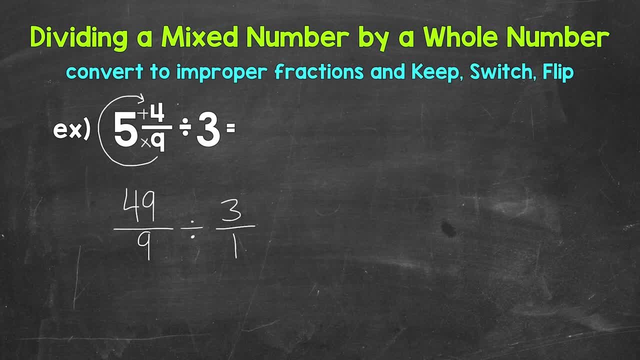 So now we have 49 9ths divided by 3 over 1.. Now let's keep switch, flip. So keep 49 9ths, Switch To multiplication And then flip 3 over 1.. So 1 is now the numerator. 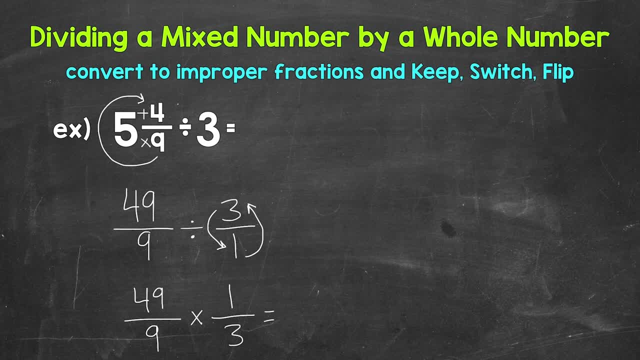 And 3 is now the denominator. So 49 9ths times 1. 3rd, Let's multiply straight across, starting with the numerators. So 49 times 1 gives us 49.. Now for the denominators: 9 times 3 gives us 27.. So we end up with 49 27ths, which is our answer. 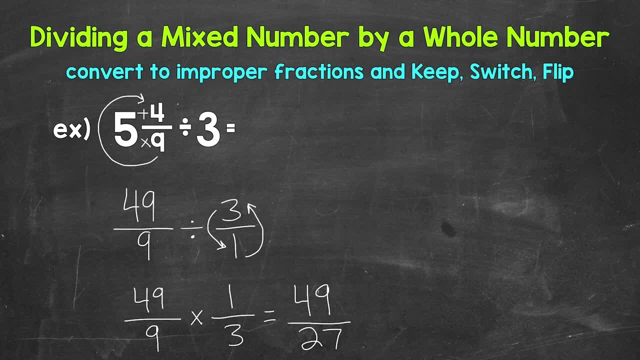 but it's an improper fraction, So let's convert it to a mixed number. We do that by dividing the numerator 49, by the denominator 27.. So 49 divided by 27.. How many whole groups of 27 in 49?? 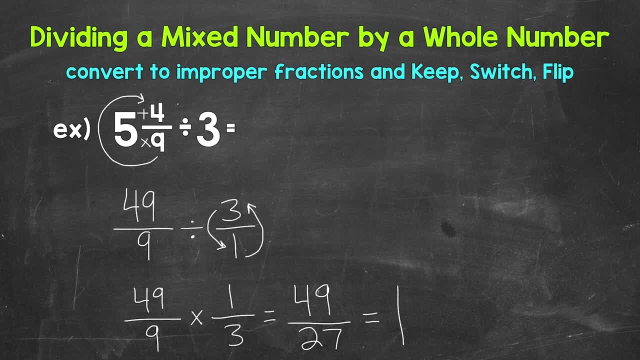 Well, 1.. Now we don't hit 49 exactly. We have a remainder, a remainder of 22.. That is the numerator of the fractional part of the mixed number, And then we keep the denominator of 27 the same, So we end up with 1 and 22 27ths. We can always look to see if we can simplify the. 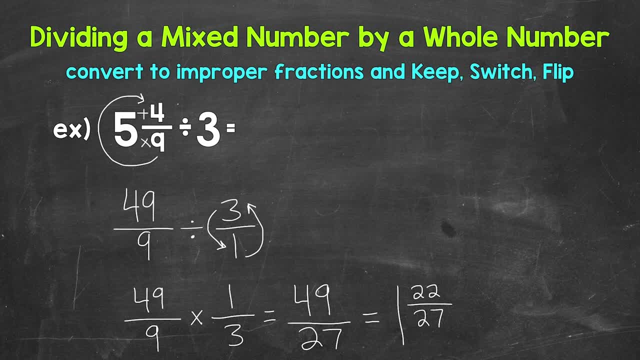 fractional part of a mixed number. The only common factor between 22 and 27 is 1.. So that is in simplest form. we are done: 1 and 22 27ths. Just for a quick recap, I'm going to write out how we went from that improper fraction of 49. 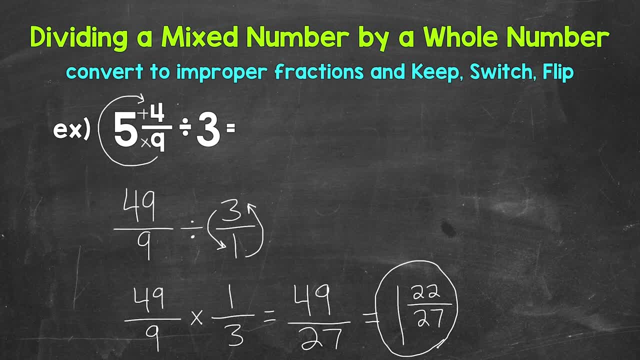 27ths to the mixed number of 1 and 22 27ths. So we divided the numerator 49, by the denominator 27.. So 49 divided by 27.. How many whole groups of 27 in 49?? Well, 1.. That is the 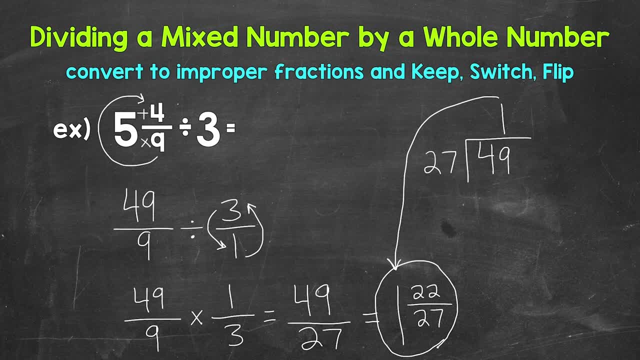 whole number of our mixed number 1 times 27 is 27.. Subtract So 49 minus 27.. 9 minus 7 is 2.. 4 minus 2 is 2 as well, So we get a remainder of 22.. 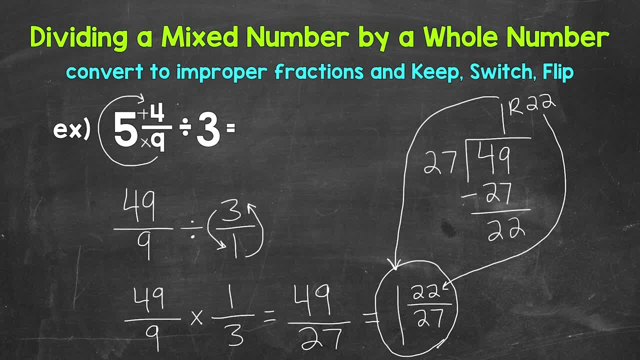 The numerator of the fractional part of the mixed number. And then we keep the denominator of 27: the same, So 1 and 22, 27ths. So there's how to divide a mixed number by a whole number. Let's move on to dividing a whole number by a mixed number. Now let's take a look at 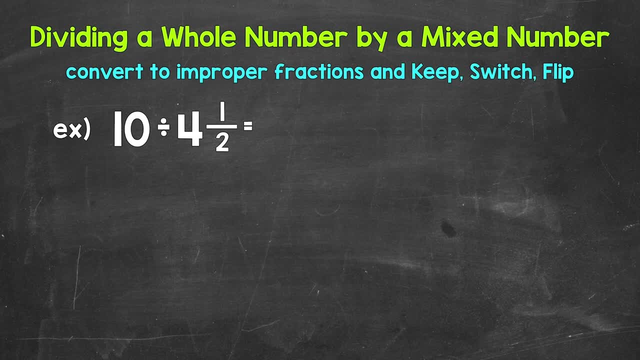 dividing a whole number by a mixed number. Let's jump into our example where we have 10 divided by 4 and a half. Now the first thing that we need to do is rewrite this problem with everything in fractional form, So everything rewritten as an improper fraction. That way we 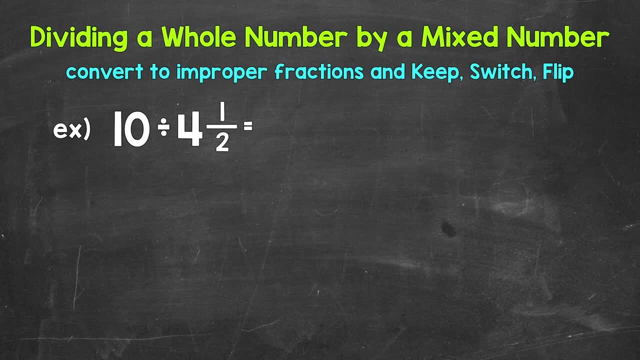 just have numerators and denominators and we can go through our steps. Keep switch flip. So let's start by rewriting 10 in fractional form, as an improper fraction, And we do that by putting it over 1.. Remember, we can rewrite any whole number in fractional form by putting it over 1. Divided by 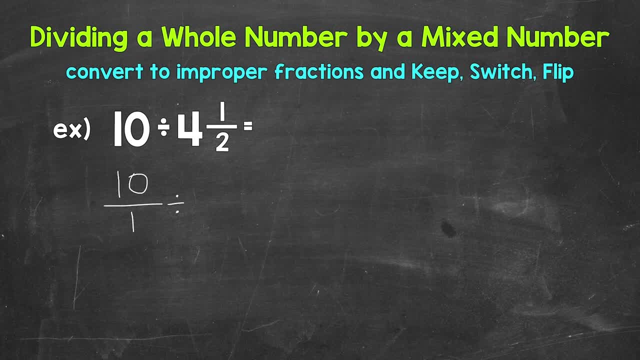 and then as far as 4 and a half. we need to convert that to an improper fraction by working our way up from the bottom. So start at the bottom and work our way up. We multiply and then add. So multiply the denominator by the whole number. So 2 times 4 is 8.. And then 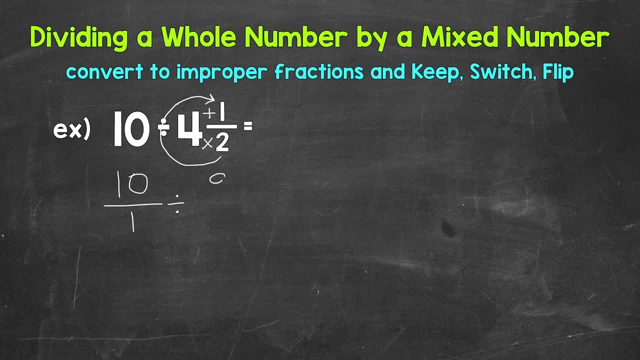 add the numerator: 8 plus 1 is 9.. That's the numerator of our improper fraction. And then keep the denominator of 2 the same, So we have 10 over 1 divided by 9 over 2.. Now we just have. 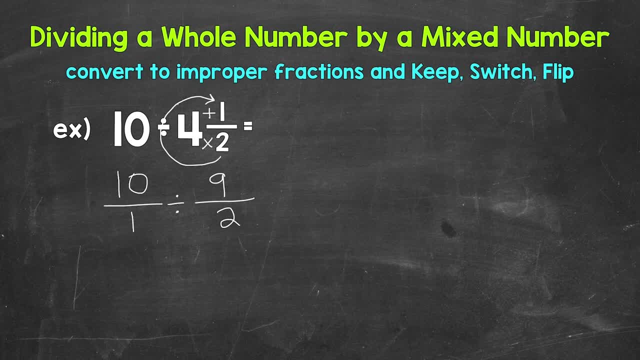 numerators and denominators and we are able to keep, switch, flip. So let's work through our steps. We keep 10 over 1., Switch to multiplication And then flip 9 over 2.. So 2 is now the numerator and 9 is now the. 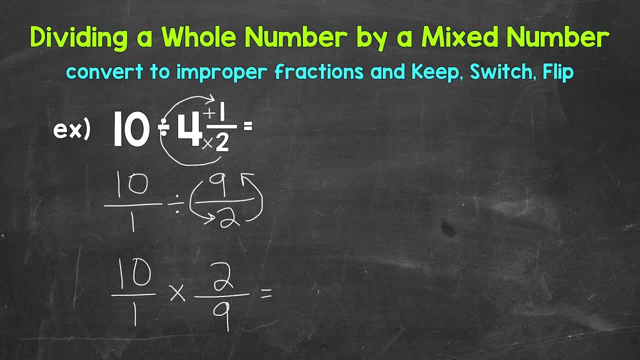 denominator. Now we can multiply straight across. Let's start with the numerators: 10 times 2 is 20.. Now for the denominators: 1 times 9 is 9.. So we end up with 29ths, Which is our. 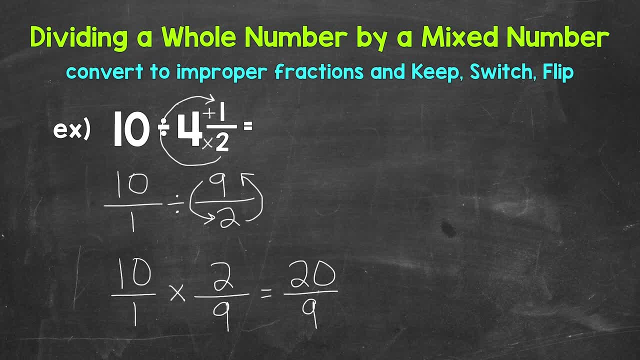 answer, But it's an improper fraction. So let's convert it to a mixed number by dividing the numerator 20 by the denominator 9.. So we have 20 divided by 9.. How many whole groups of 9 in 20?? 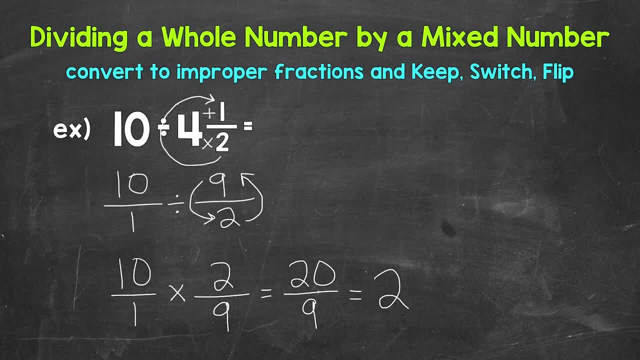 Well, 2 whole groups of 9 in 20.. That's the whole number of our mixed number. Now we don't hit 20. exactly 2 whole groups of 9 gets us to 18.. So we have a remainder of 9 divided by 9.. To that function we remove 1. And after we get, notamment, 8,. 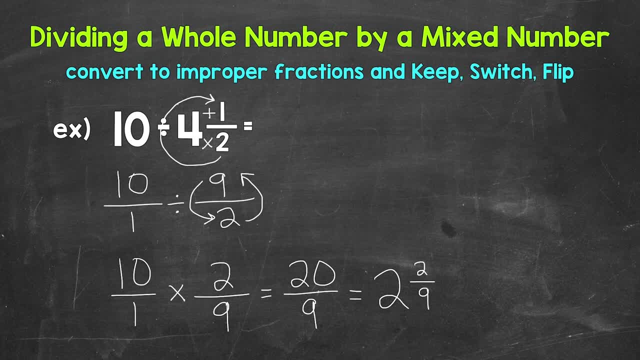 2. That is the numerator of the fractional part of the mixed number, And then we keep the denominator of 9 the same, So we end up with 2 and 2 9ths. We can always look to see if we can. 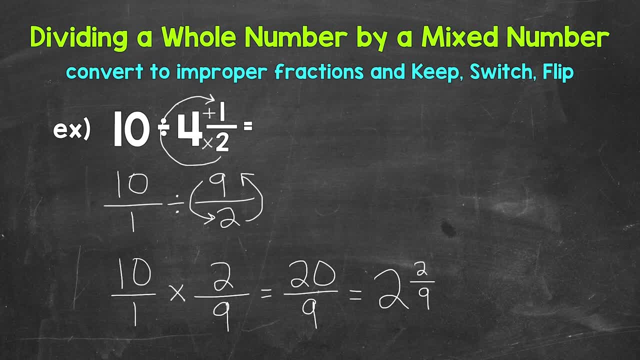 simplify the fractional part of a mixed number. The only common factor between 2 and 9 is 1.. So this is in simplest form and we are done: 2, 9ths. Now I do want to go through a quick recap as far as how we went from that improper fraction. 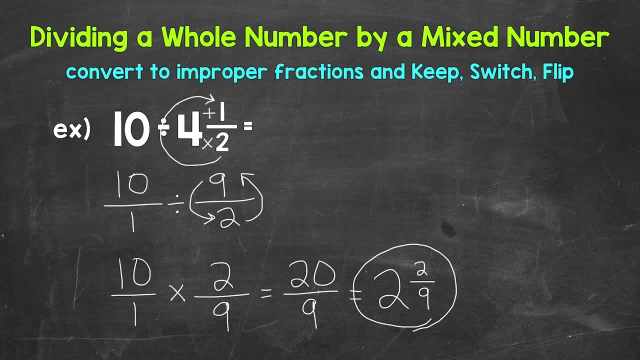 of 20 9ths to the mixed number of 2 and 2 9ths. So again we divided the numerator 20.. So I'm going to write this out off to the side here. So numerator 20 divided by the denominator 9.. So how? 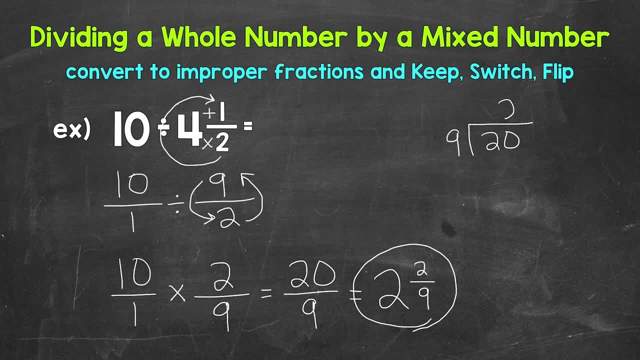 many whole groups of 9 and 20?? 20 divided by 9.. Well, 2, and that 2 is the whole number of the mixed number. Now we multiply 2 times 9 is 18.. Subtract 20 minus 18 is 2.. So we get a remainder of 2.. 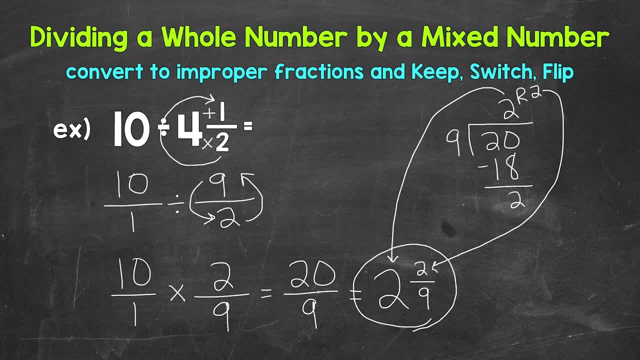 That remainder is the numerator of the fractional part of the mixed number, and then we keep the denominator of 9.. The same, So there's how to divide a whole number by a mixed number. Let's move on to dividing a mixed number by a fraction. Now let's take a look at dividing a mixed number by a fraction. 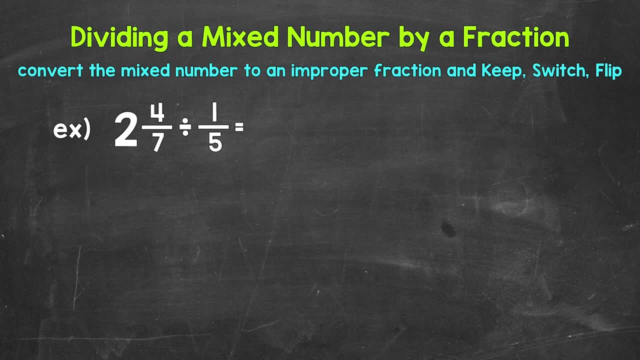 Let's jump into our example where we have 2 and 4 7ths divided by 1- 5th. Now the first thing that we need to do is convert the mixed number to an improper fraction. That way, we just have a numerator and a denominator. So we have a numerator and a denominator. So we have a numerator and a. 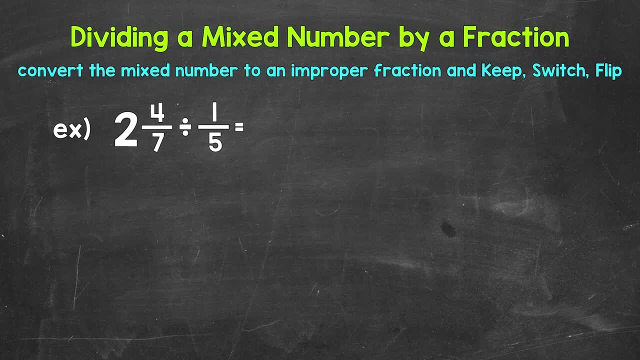 denominator and we can go through our dividing fractions. steps Keep switch flip. So let's convert 2 and 4, 7ths to an improper fraction. So we start at the bottom, We multiply and then add, So the denominator times the whole number. 7 times 2 is 14 and then add the numerator 14 plus 4 is 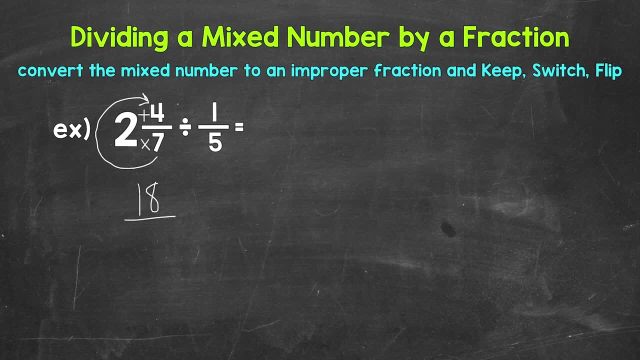 18.. That is our numerator of the improper fraction. And then we keep the denominator of 7, the same Divided by 1, 5th. So I rewrote the problem with the mixed number as an improper fraction. Now let's go. 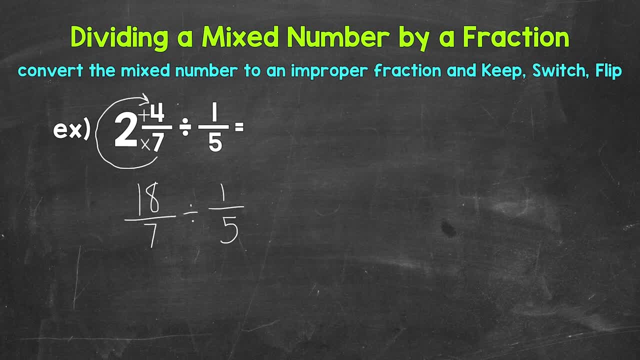 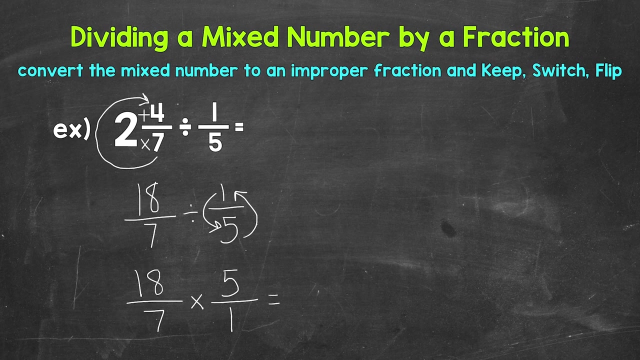 through our steps: Keep, switch, flip. So keep 18- 7ths, Switch to multiplication And then flip 1- 5th. So 5 is now the numerator and 1 is now the denominator. Now we can multiply straight across. Let's start with the numerators: 18 times 5, that gives us 90.. 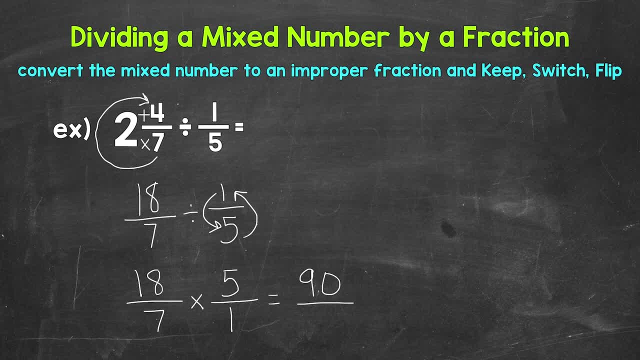 Now for the denominators: 7 times 1,, that gives us 7.. So we end up with 90 7ths, Which is our answer for the denominator. So we can multiply straight across. Let's start with the numerators: 18 times 5,, that gives us 90.. 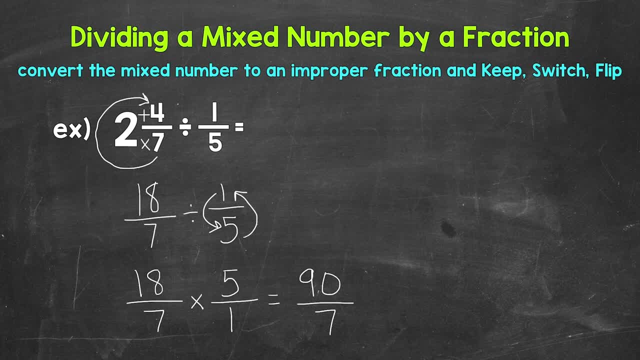 But it's an improper fraction, So let's convert it to a mixed number. We do that by dividing the numerator 90, by the denominator 7.. So we have 90 divided by 7.. So how many whole groups of 7 in? 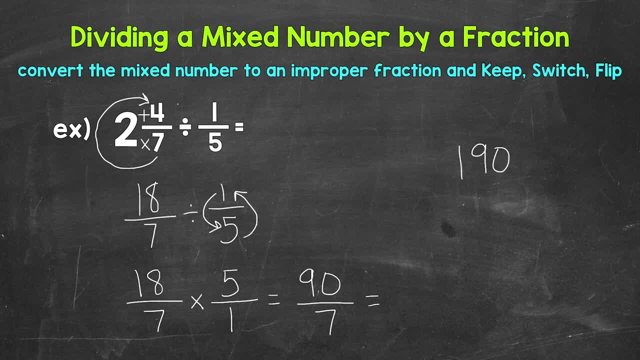 90?? Well, let's work through this off to the side here. So 90 divided by 7.. 9 divided by 7. We have 1. 1 whole group of 7 in 9.. Multiply 1 times 7 is 7. Subtract. 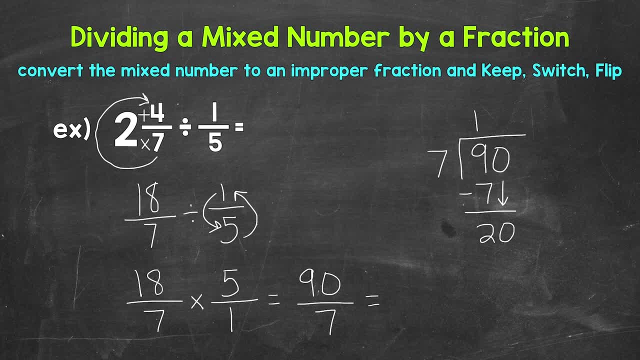 9 minus 7 is 2. Bring down. And now we repeat. So we divide 20 divided by 7.. How many whole groups of 7 in 20?? Well, 2. 2 times 7 is 14.. Subtract 20 minus 14 gives us a remainder of 6. So 12 whole. 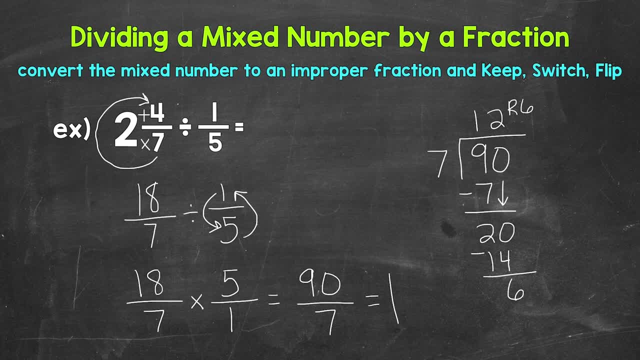 groups of 7 in 90. That's the whole number of 7.. So we divide 20 divided by 7.. How many whole groups of 7 in 20?? Well, 2. 2 times 7 is 14.. Subtract 20 minus 14 gives us a remainder of 6.. So 12 whole. 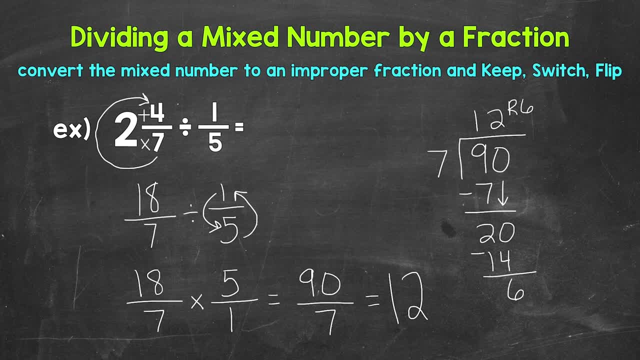 groups of 7 in 20.. That's the whole number of 7.. Subtract 20 minus 14 gives us a remainder of 6. We don't hit 90 exactly. That remainder is the numerator of the mixed number, And then we keep. 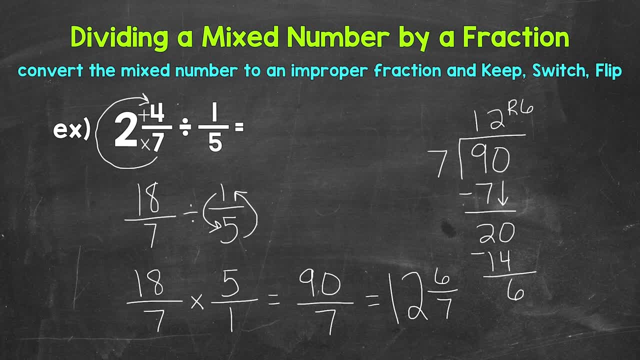 the denominator of 7 the same, So we end up with 12 and 6 sevenths. We can always look to see if we can simplify the fractional part of a mixed number. 6 sevenths is, in simplest form, the only. 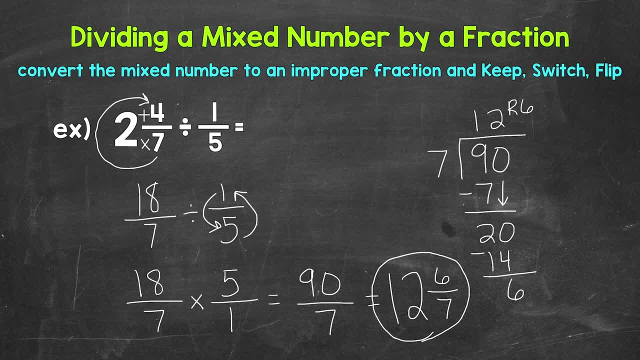 common factor between 6 and 7 is 1.. So we are done: 12 and 6 sevenths. So there's how to divide a mixed number by a fraction. Let's move on to dividing a fraction by a mixed number. Now let's 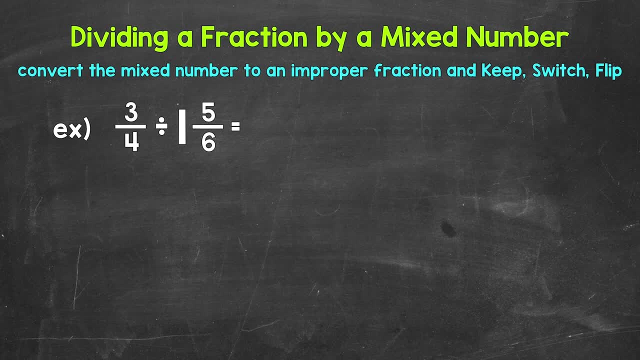 take a look at dividing a fraction by a mixed number. Let's jump into our example where we have 3 fourths divided by 1 and 5 sixths. Now the first thing that we need to do is rewrite this problem with the mixed number written as an improper fraction. So we need to 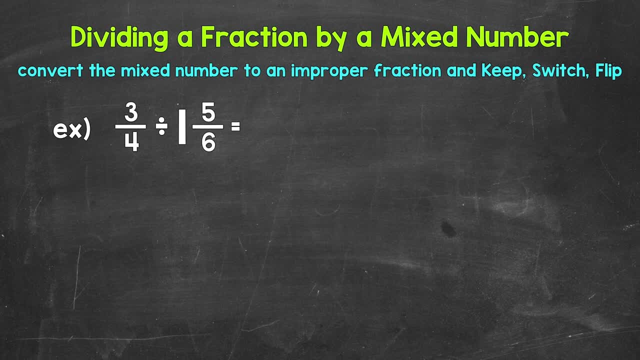 convert that mixed number to an improper fraction. That way we just have numerators and denominators and we can go through our steps, Keep switch flip. So let's rewrite this problem. We have 3 fourths divided by, and then as far as 1 and 5 sixths, let's convert. 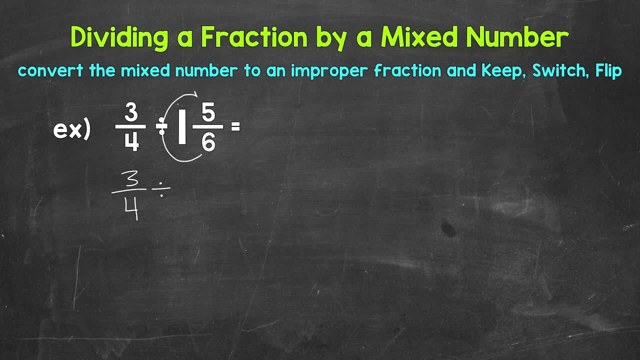 this to an improper fraction. We start at the bottom and work our way up. We multiply and then add. So take the denominator and multiply it by the whole number. So 6 times 1 is 6.. And then add the numerator: 6 plus 5 gives us 11.. That's the numerator of the improper fraction. And then we 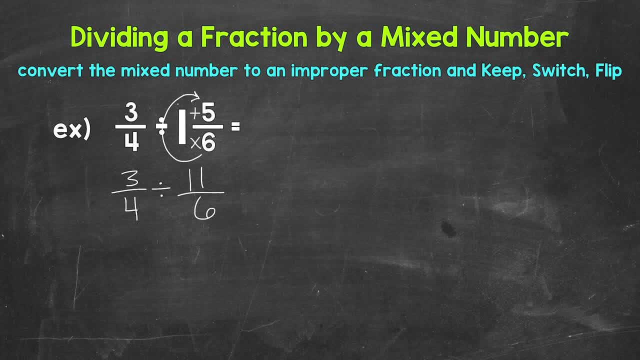 keep the denominator of 6 the same. So now we have 3 fourths divided by 1 and 5 sixths. Now let's go through our steps: Keep, switch flip. So keep 3 fourths. Switch to multiplication. 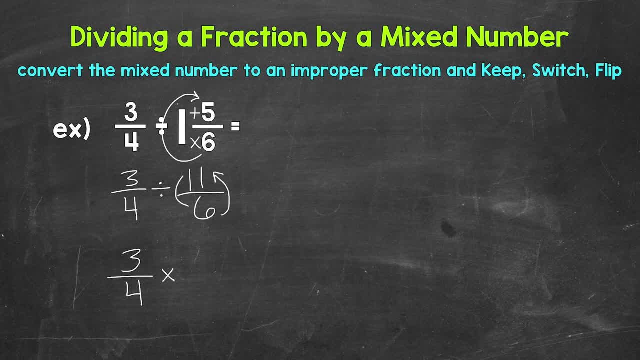 And then flip 11- sixths. So 6 is now the numerator And 11 is now the denominator. So we have 3 fourths times 6 elevenths. Now let's multiply straight across, Starting with the denominator. So we have 3 fourths times 6 elevenths, And then flip 11- sixths, So 6 is now. 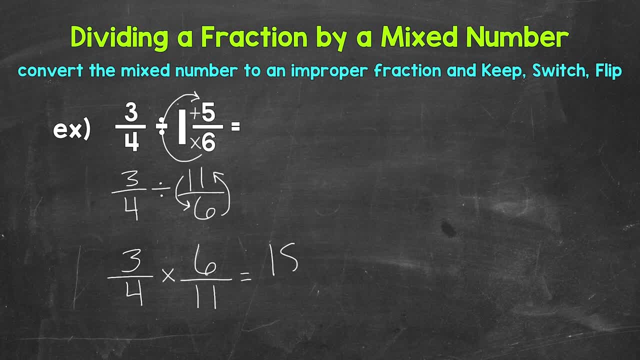 the numerator. So 3 times 6 is 18.. Now for the denominators: 4 times 11 is 44. So we get 18 forty-fourths, Which is our answer. but we can simplify this fraction. We have a common factor. 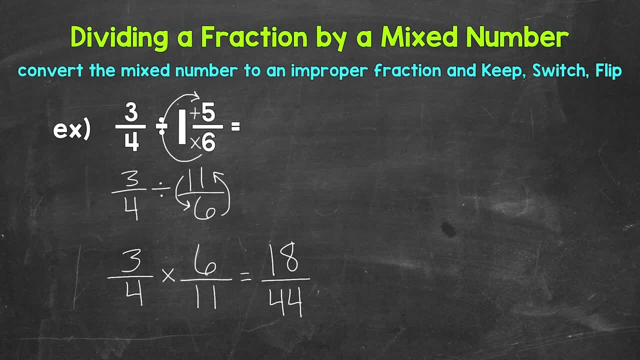 other than 1 between 18 and 44. We have a greatest common factor of 2.. So let's divide 18 by 2. And 44 by 2.. 18 divided by 2 is 9.. 44 divided by 2 is 22.. So we end up with 9 twenty-seconds. 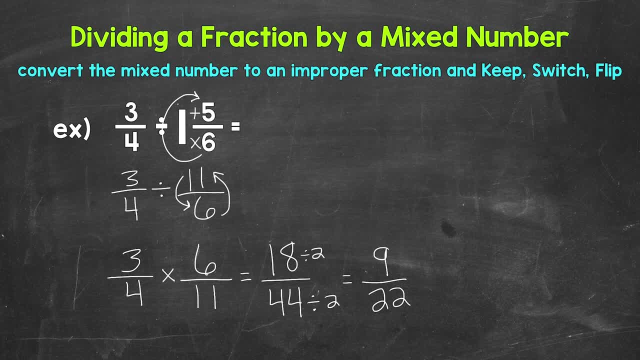 or 9 over 22.. The only common factor between 9 and 22 is 1.. So this is in simplest form And we are done. So there's how to divide a fraction by a mixed number. Let's move on to. 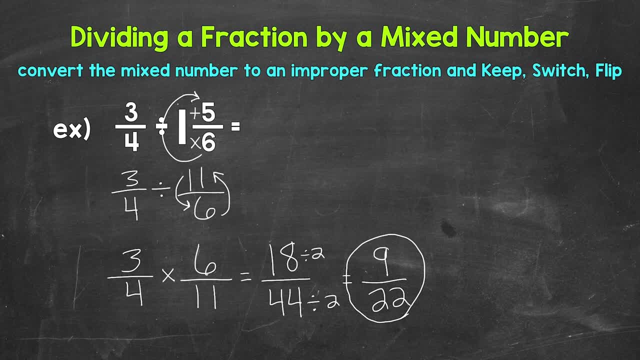 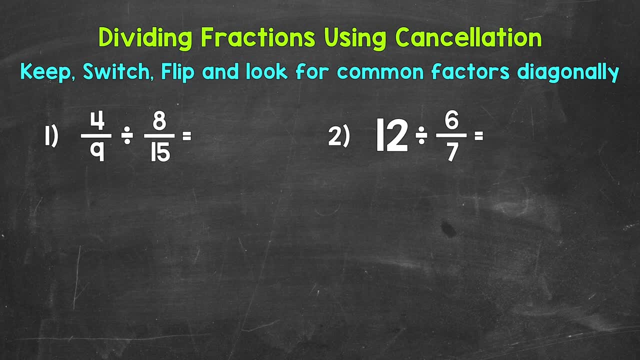 using cross-cancellation when we have a division problem involving fractions. Now we will take a look at using cross-cancellation when we have a division problem involving fractions. Cancellation gives us smaller numbers in value to work with and easier numbers to work with. This is a way 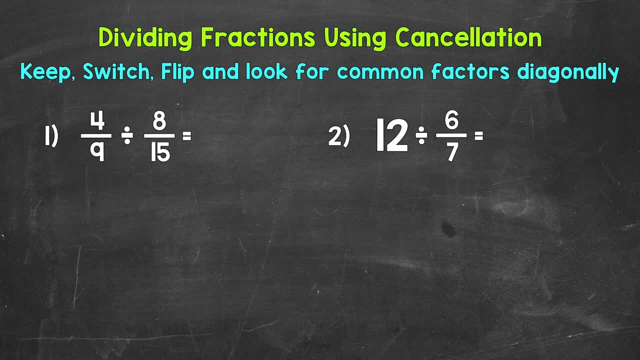 to simplify the problem before multiplying And remember when we have a division problem involving fractions, we end up multiplying. Let's jump into number one, where we have 4 ninths divided by 8 fifteenths We can't use. 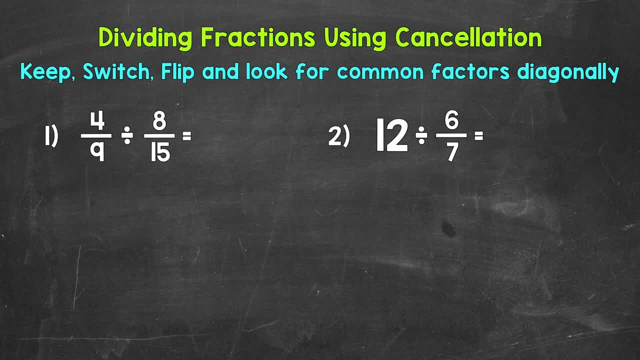 cancellation quite yet. We can't use it right away. We use cancellation when multiplying fractions. So we need to wait until we go through the steps we use to divide fractions: Keep, switch flip Or keep change flip. So let's keep the first fraction of 4 ninths. 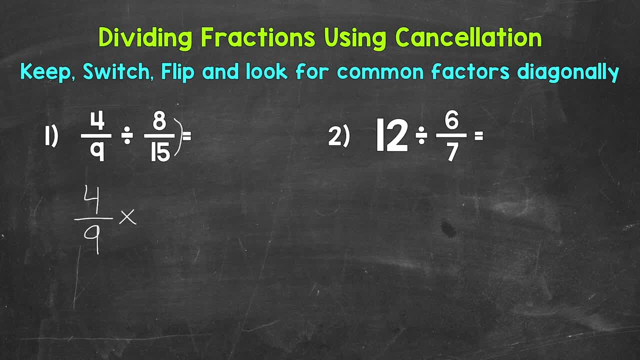 Switch to multiplication and then flip the second fraction of 8 fifteenths. So 15 is now the numerator and 8 is now the denominator. Now we can multiply straight across, But before doing so, we can look to use cancellation. When we use cancellation, we look diagonally. 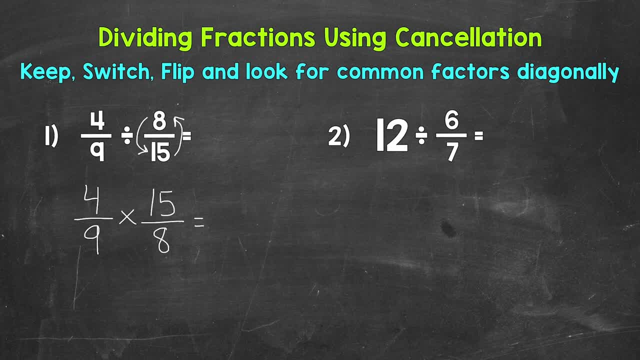 for common factors other than 1 that we can divide by. This is like simplifying fractions, but we are looking diagonally. So for number 1, we look at 4 and 8, and then 9 and 15.. Let's look at 4 and 8 first. Are there any common? 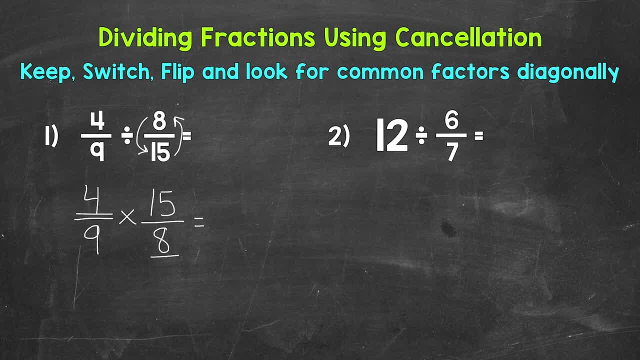 factors other than 1, that we can divide 4 and 8 by. Yes, Let's use the greatest common factor of 4.. So we can divide 4 and 8 by 4.. 4 divided by 4. Is 1.. 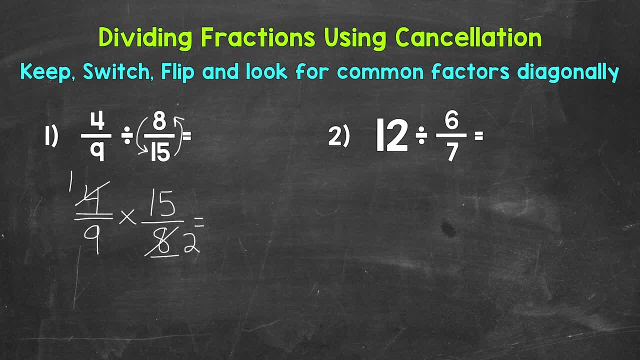 8 divided by 4. Is 2.. Now we can take a look at 9 and 15.. Are there any common factors other than 1 that we can divide 9 and 15 by? Yes, 3 is a common factor between 9 and 15. And it's the greatest common. 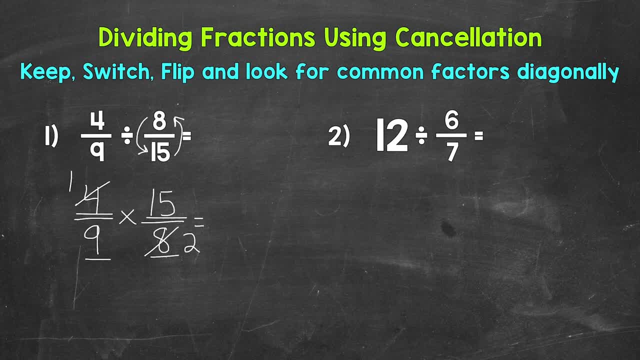 factor. So let's divide 9 and 15 by 3.. 9 divided by 3 is 3.. 15 divided by 3 is 3.. divided by 3 is 5.. Now we can multiply straight across and we have smaller numbers in value. to. 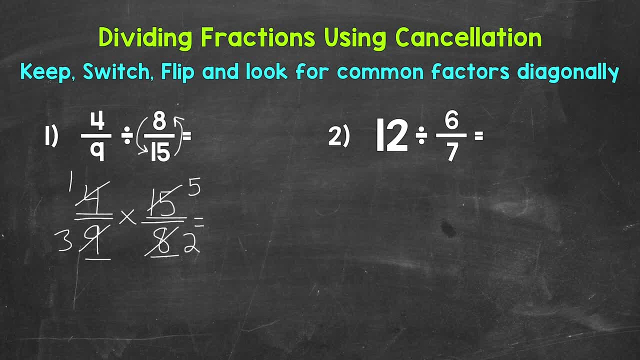 work with Easier numbers to work with. Let's start with the numerators: 1 times 5 is 5.. Now for the denominators: 3 times 2 is 6.. So we end up with 5, sixths, The greatest common factor. 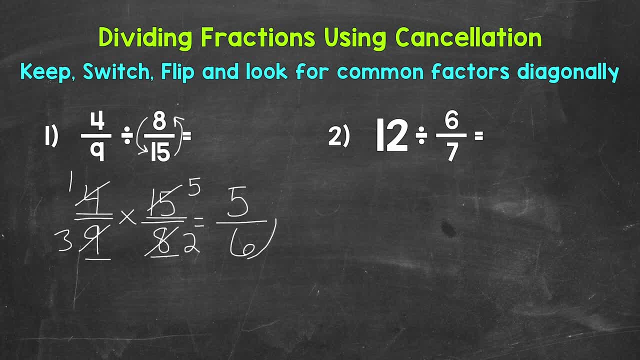 between 5 and 6 is 1.. So we are in simplest form, and this is our final simplified answer. Again: 5, sixths. Now let's work through that problem without using cancellation and see what happens. So keep, switch, flip. So keep 4, ninths, Switch to multiplication and then flip 8, 15ths. So now we 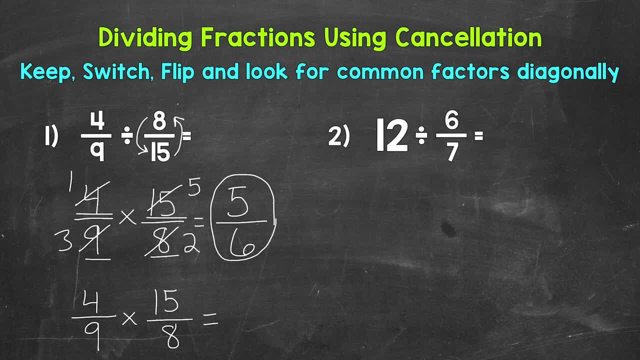 have 15 eighths. Let's multiply straight across: 4 times 15 is 60.. 9 times 8 is 72.. So we get 60- 70 seconds. Now that's different than the answer above. That's because we haven't simplified yet. Are there any common? 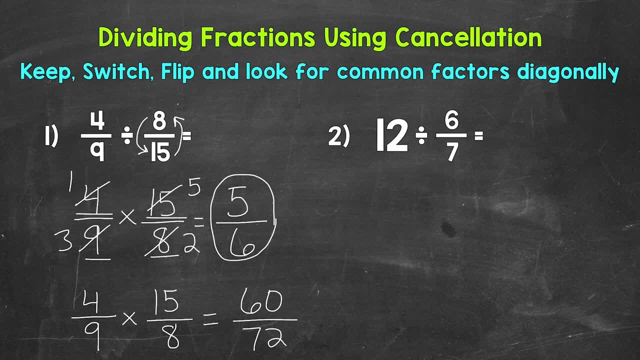 factors between 60 and 72 other than 1?? Yes, The greatest common factor between 60 and 72 is 60. 12.. So let's divide both of them by 12.. 60 divided by 12 is 5.. 72 divided by 12 is 6.. So you can see. 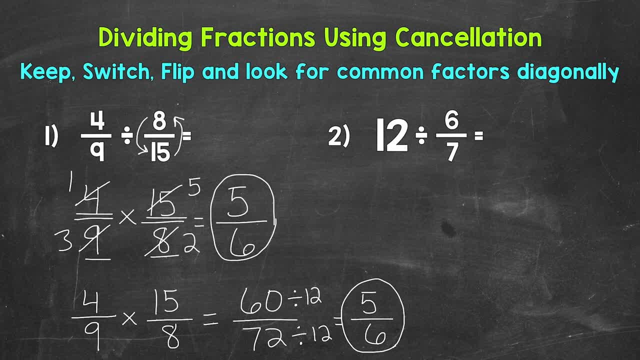 that we get 5 sixths. that way as well, We get the same answer either way. Now do we have to use cancellation? No, But it's a good strategy to be familiar with and use. when possible It can be helpful. Let's move on to number 2, where we have 12 divided by 6 sevenths. Let's keep switch flip, So keep. 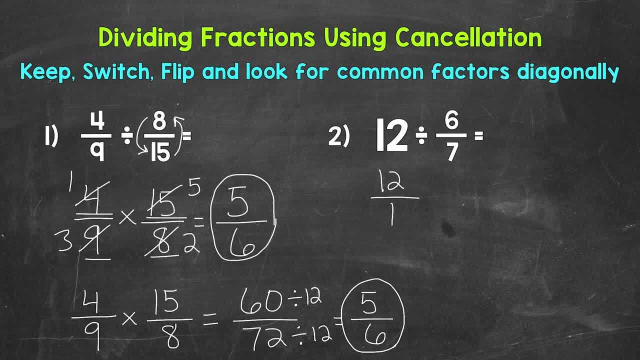 12, and I'm going to write it in fractional form. That way we have a numerator and a denominator and we can multiply straight across. Remember, we can rewrite any whole number in fractional form by putting it over 1. Then we can switch to multiplication and flip. 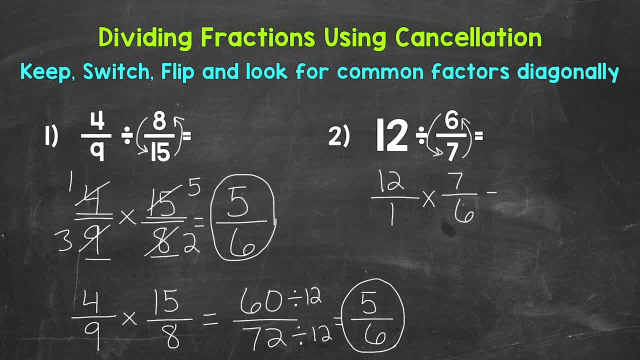 So 7, sixths. Now we can multiply straight across, but before doing so we can look to use cancellation. So let's look diagonally for common factors other than 1.. Let's look at 12 and 6 first. Are there any? 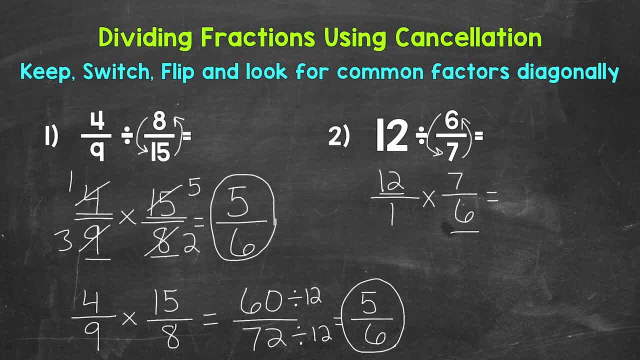 common factors other than 1 that we can divide by. Yes, 6 is the greatest common factor between 12 and 6.. So let's divide by 6.. 12 divided by 6 is 2.. 6 divided by 6 is 1.. Now let's take a look at 1 and 7.. Are there any common? 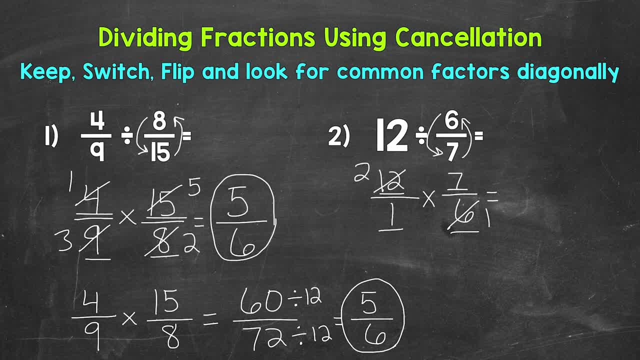 factors between 1 and 7 other than 1 that we can divide by No. So we can't use cancellation going that way. So now we're ready to multiply straight across. Let's start with the numerators: 2 times 7. 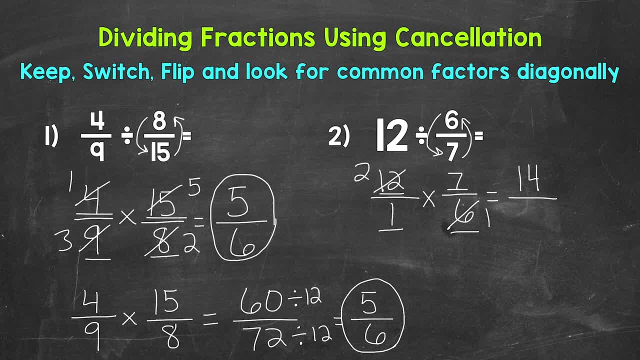 is 14.. Now for the numerator: 2 times 7 is 14.. Now for the denominator: 2 times 7 is 14.. Now for the denominators: 1 times 1 is 1.. So we end up with 14 over 1, which is 14.. And that's our final answer. 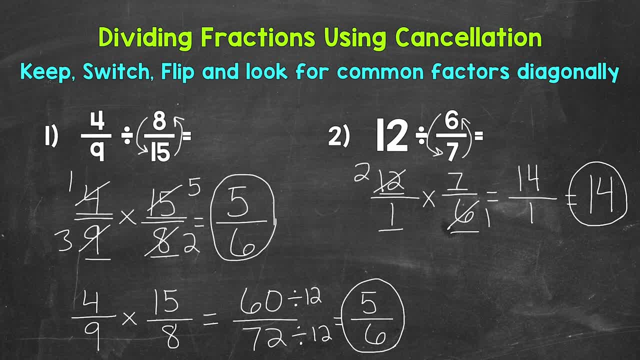 So there you have it. There's how to use cancellation when we have a division problem involving fractions. Now can we use cancellation with every single problem? No, We have to have common factors other than 1 that we can divide by diagonally. And do we have to? 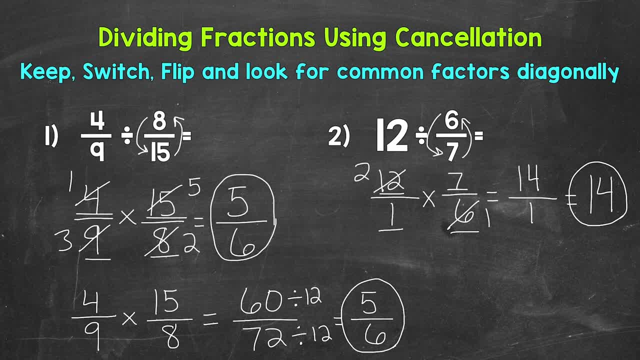 to use cancellation in order to get to the correct answer? No, but it is a good strategy to be familiar with and it can be helpful. So there's how to use cross cancellation. when we have a division problem involving fractions, Let's move on to using cross cancellation when dividing mixed. 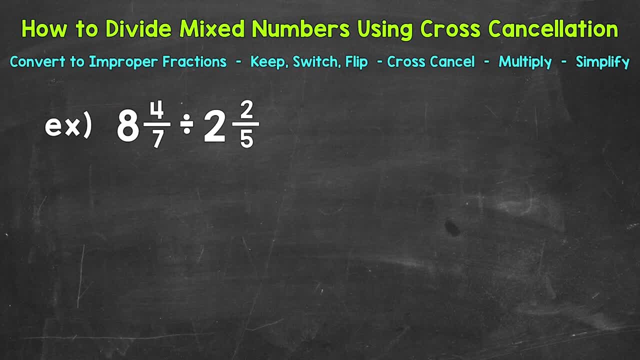 numbers. Now we will take a look at using cross cancellation when dividing mixed numbers. Let's jump into our example where we have 8 and 4 7ths divided by 2 and 2 5ths. Now we use cross cancellation when we get to the multiplying step. So keep that in mind. Now, the first thing that we 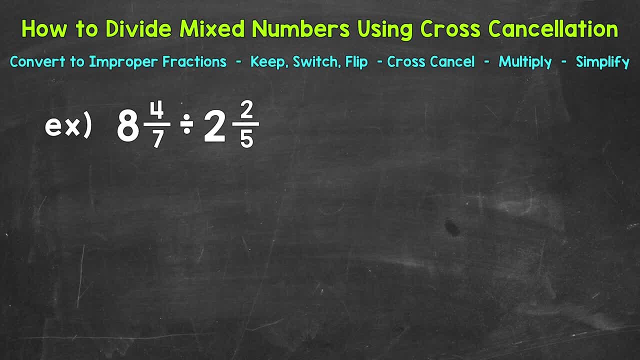 want to do is convert these mixed numbers to improper fractions. That way we just have a numerator and a denominator and we can move forward with our steps. So we'll start with 8 and 4 7ths. we'll start at the bottom and work our way to the top. We multiply, then add, So we do our. 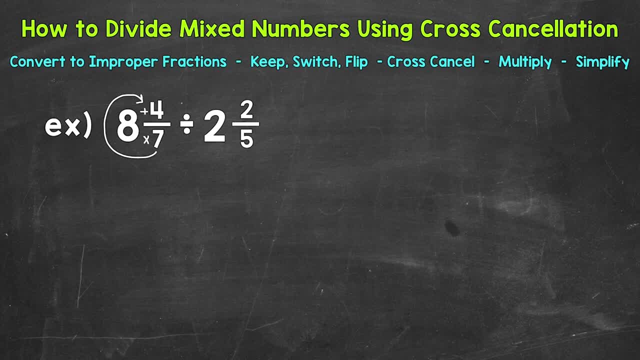 denominator times the whole number. 7 times 8 is 56 plus our numerator of 4.. So 56 plus 4, that gives us 60. We keep our denominator of 7 the same. Let's bring our division sign down, then do the second. 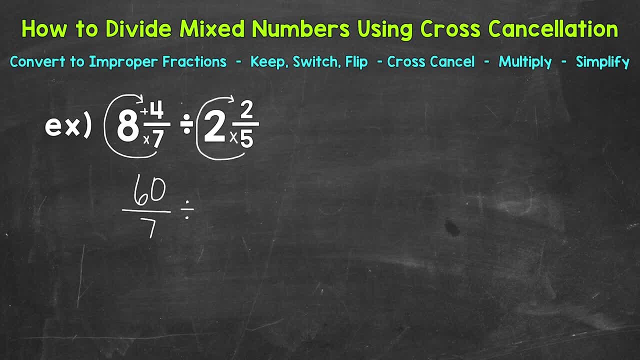 mix number here. So start at the bottom, multiply, then add 5 times 2 is 10 plus 2 is 12.. So we get 12 5ths. Now that we have our mixed numbers converted to improper fractions, we can go. 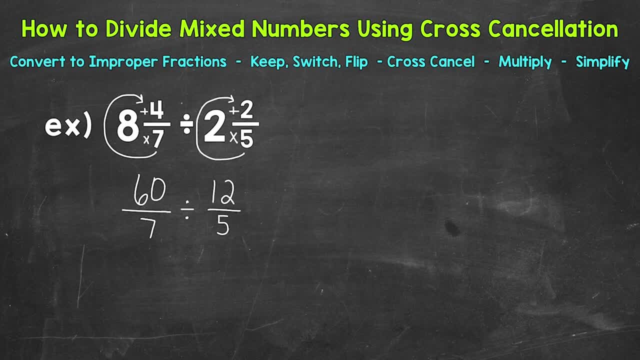 through our dividing fractions steps: Keep switch flip, Also known as keep change flip. There's different words out there for the steps, But they all mean the same thing. One thing I do want to mention before moving forward: these improper fractions are equivalent to the mixed numbers. So 60 7ths is equivalent to 8, and 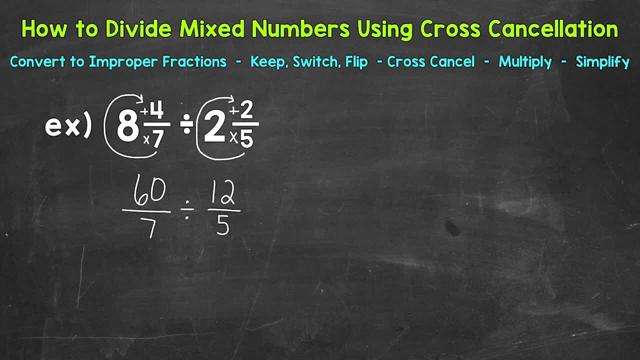 4, 7ths, 12, 5ths is equivalent to 2 and 2- 5ths. So when we convert to improper fractions, we're not changing the value of the problem at all. All right, let's go through our steps. keep switch flip. 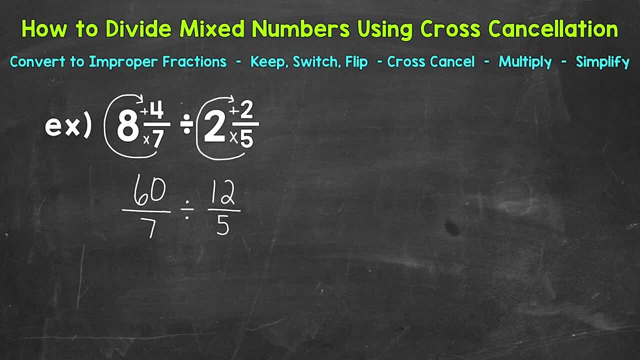 So we always keep the first fraction, so 60 over 7. then we switch or change to multiplication and then flip our second fraction, So the denominator becomes the numerator and the numerator becomes the denominator. this is called the reciprocal. so we have 5 12ths. Now we can multiply. 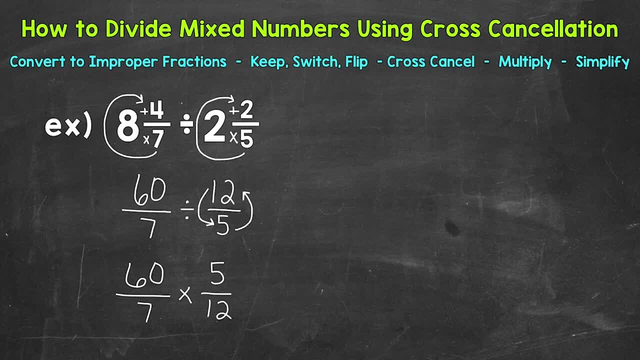 straight across. but in this problem we have an opportunity for cross-cancellation. Cross cancellation is a way to simplify fractions before multiplying. It gives us smaller and easier numbers to work with, therefore a simpler problem to solve. We cross cancel by looking for common factors between the numerators and denominators, so the top and bottom. 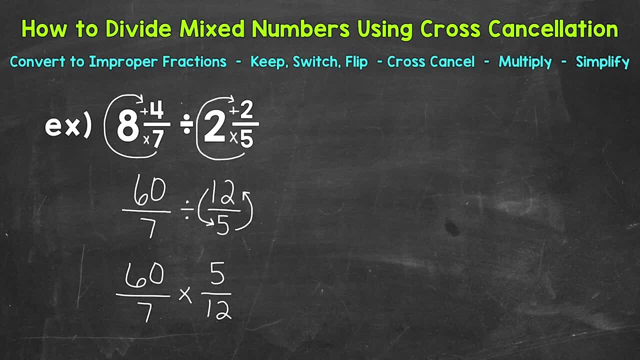 Think of it like simplifying fractions, but we can look diagonally as well. For example, we have common factors other than 1, between 60 and 12, and a greatest common factor of 12.. So let's divide 60 and 12 by 12.. 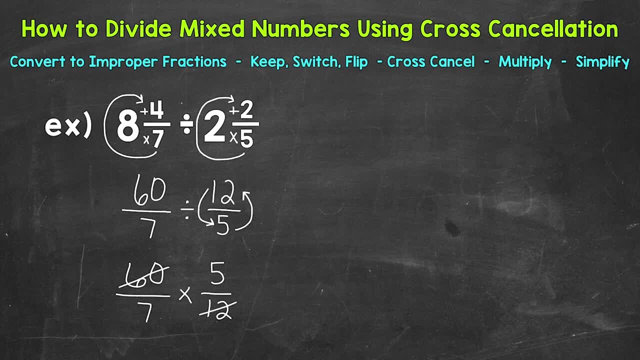 We do that by crossing them out and dividing by 12.. So 60 divided by 12 is 5.. 12 divided by 12 is 1.. We can also look diagonally the other way, so we have 7 and 5.. 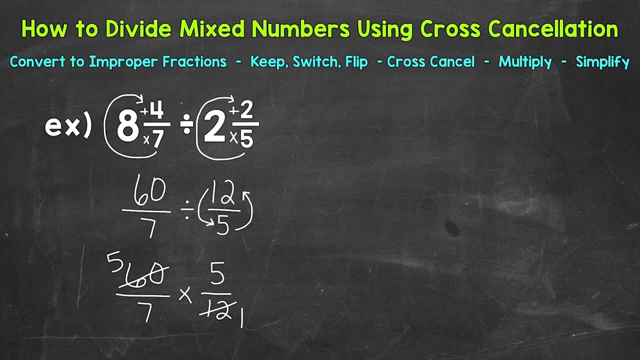 The only common factor between 7 and 12 is 1.. 7 and 5 is 1, so we can't use cross cancellation with the 7 and the 5.. Once we cross cancel, we can multiply straight across. So we have 5 times 5,, which is 25.. 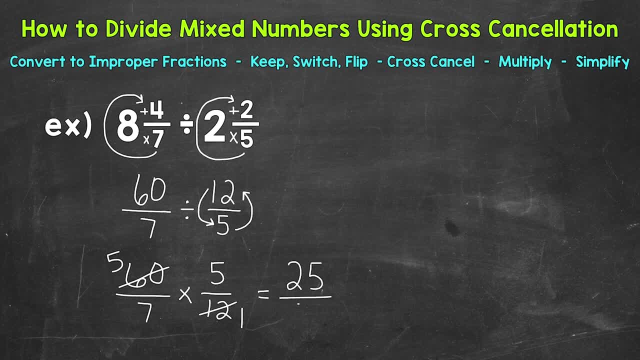 And then we have 7 times 1, which is 7.. So we get to 25 sevenths. That's an improper fraction. Let's convert it to a mixed number. So we do that by doing the numerator 25, divided by 7.. 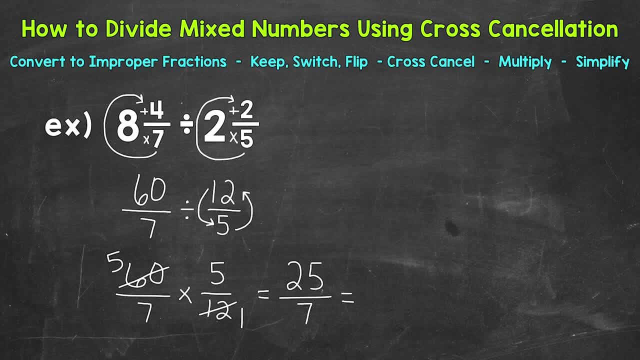 So 25 divided by 7, let's think: how many whole groups of 7 can we pull out of 25?? Well, 3 whole groups of 7, that's our whole number. Now we do not hit 25 exactly. we have something left over, a remainder. 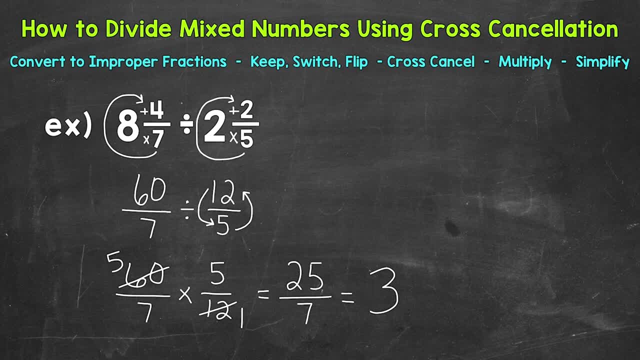 So the difference between 25 and 21 is 4, that's our remainder, So that's our numerator, and then we keep our denominator of 7 the same. Always. look to see if you can simplify this, If you want to simplify the fractional part of a mixed number. 4, sevenths is in simplest form: 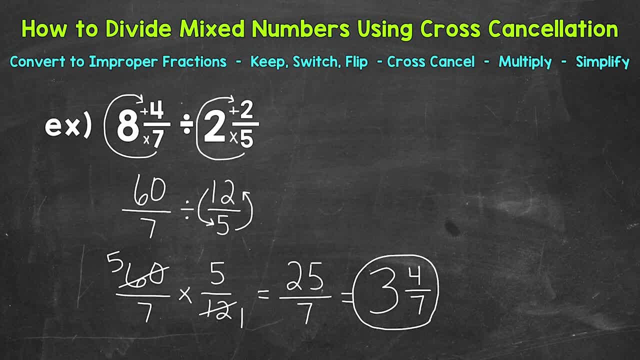 So this is our final answer. 3 and 4, sevenths: Now do we have to use cross cancellation? No, we can multiply straight across and do 60 times 5 and 7 times 12, then go from there. But cross cancellation again gave us smaller and easier numbers to work with. 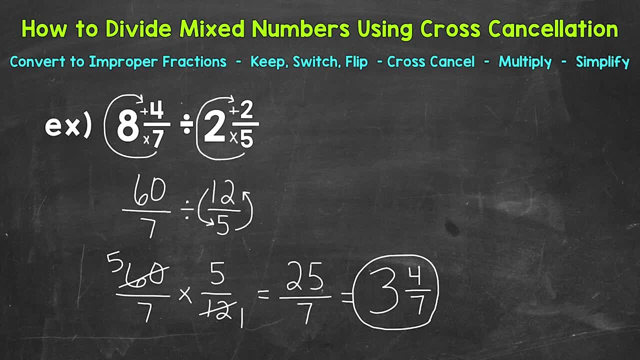 It's a useful tool. It's a tool to use when looking at multiplication problems that involve fractions. And another thing I want to mention: cross cancellation can't be used with every problem. We have to have common factors other than 1 between our numerators and denominators that we can divide by. 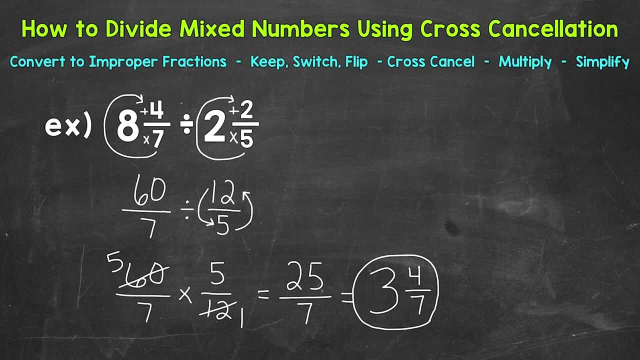 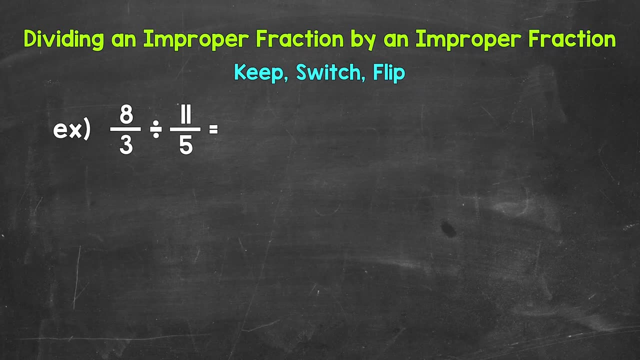 If the only common factor is 1,, then cross cancellation cannot be used. So there's how to use cross cancellation when dividing numbers. Let's move on to dividing improper fractions by improper fractions. Now we can take a look at dividing an improper fraction by an improper fraction. 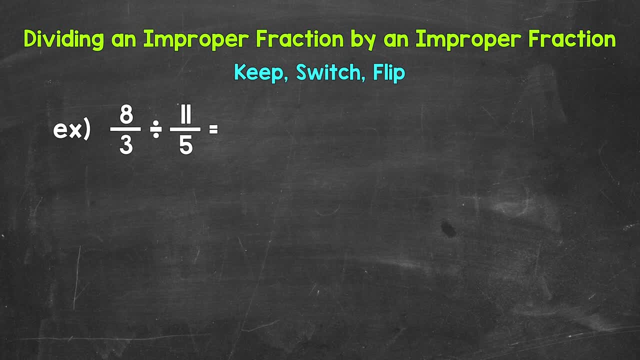 Now, when we have a division problem involving improper fractions, we go through the same steps we use when we have division problems involving proper fractions: Keep switch flip. So don't let a problem hold you up. if it involves improper fractions, Keep switch flip. 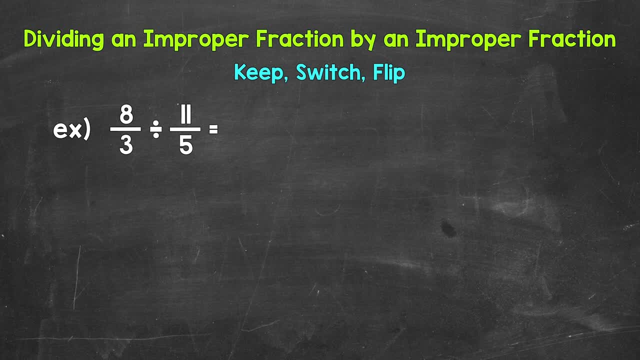 So don't let a problem hold you up if it involves improper fractions. Again, just go through the same steps. Let's jump into our example where we have 8 thirds divided by 11 fifths, So keep, switch, flip. So keep 8 thirds, switch to multiplication and then flip 11 fifths. 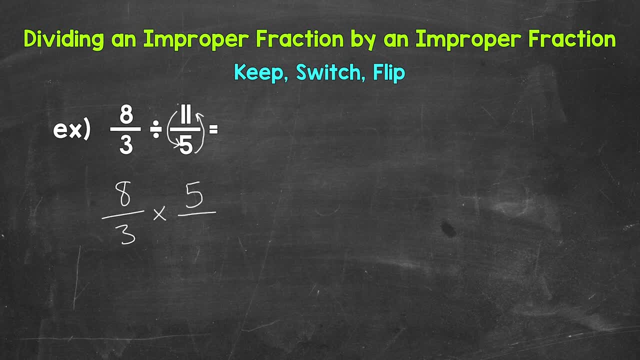 So 5 is now the numerator And 11 is the numerator And 11 is now the denominator. Now we can multiply straight across. Let's start with the numerators: 8 times 5 is 40.. Now for the denominators. 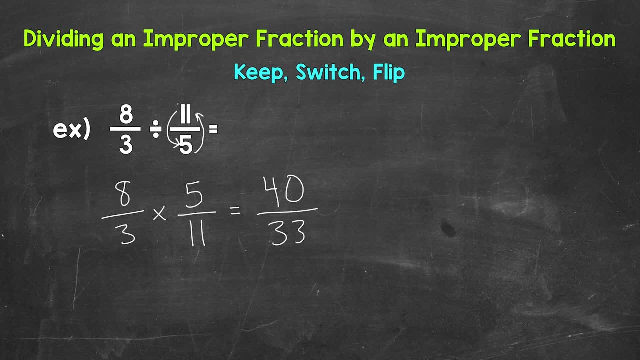 3 times 11 is 33.. So we end up with 40 over 33, or 40 thirty-thirds. Now, that is our answer, but it's an improper fraction, So let's convert it to a mixed number by dividing. 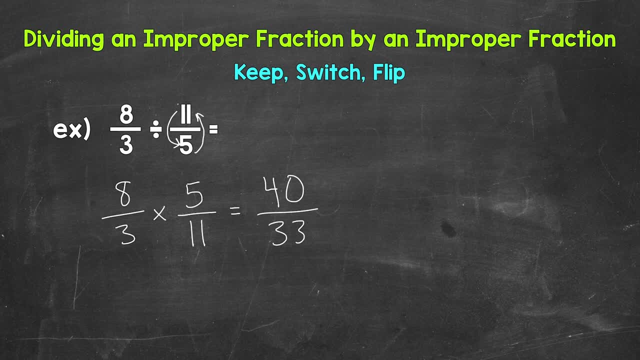 The numerator 40, by the denominator 33.. So how many whole groups of 33 in 40?? Well, one whole group of 33 in 40. Now we don't hit 40 exactly. We have a remainder. 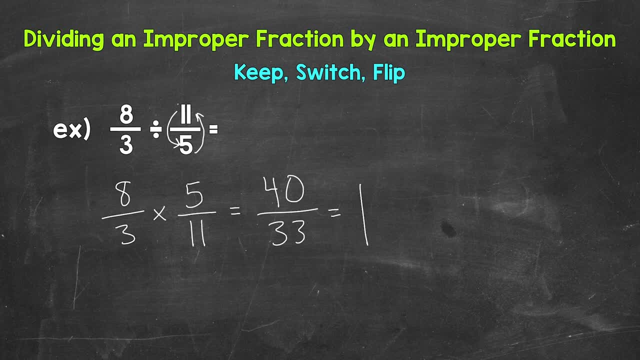 And that remainder is 7.. That's the numerator of the fractional part of the mixed number. And then we keep the denominator of 33, the same. Always look to see if you can simplify The fractional part of a mixed number. 7 thirty-thirds is in simplest form. the only common factor between 7 and 33 is 1.. 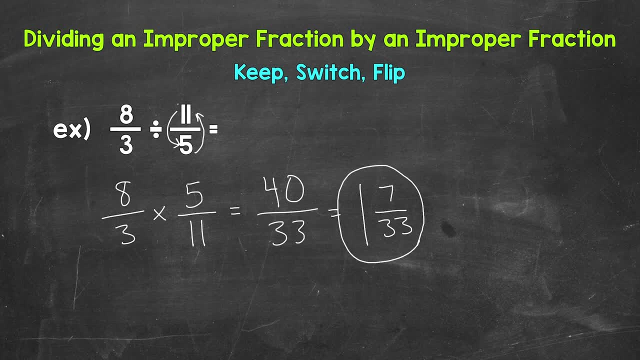 So this is our final answer: 1 and 7 thirty-thirds. Now, just as a quick recap as far as how we went from that improper fraction of 40 over 33 to the mixed number of 1 and 7 thirty-thirds, I'm going to write it down: 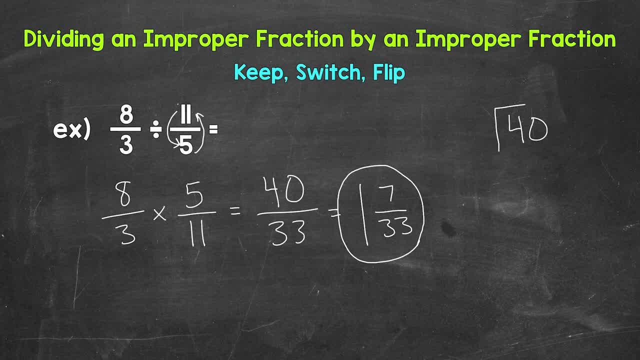 So again, we divided the numerator 40, by the denominator 33.. So 40 divided by 33.. How many whole groups of 33 in 40?? Well, 1. 1 times 33 is 33.. 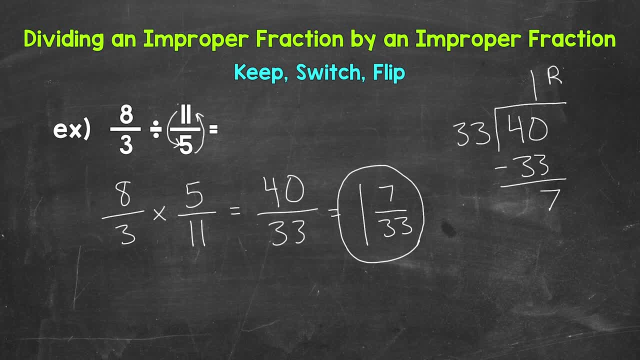 Subtract And we get that remainder of 7.. 1 is the whole number, part of the mixed number, And then 7.. The remainder is the numerator of the fractional part, And then we keep the denominator of 33 the same. So there's how to divide an improper fraction by an improper fraction. 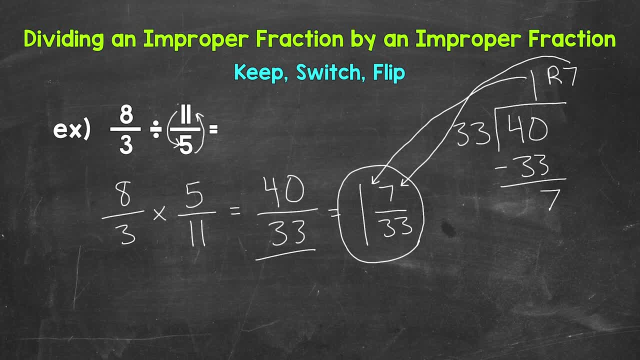 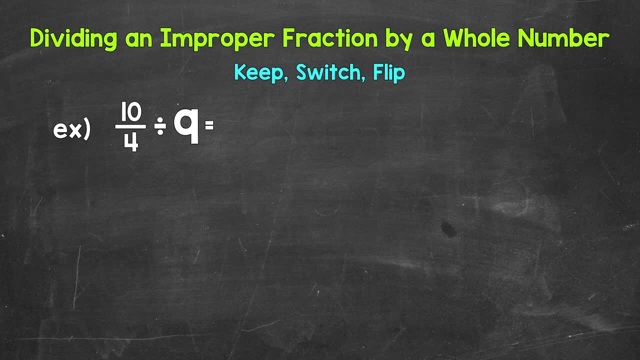 Let's move on to dividing an improper fraction by a whole number. Now we will take a look at dividing an improper fraction by a whole number. Let's jump into our example where we have 10 fourths divided by 9.. So keep switch flip. 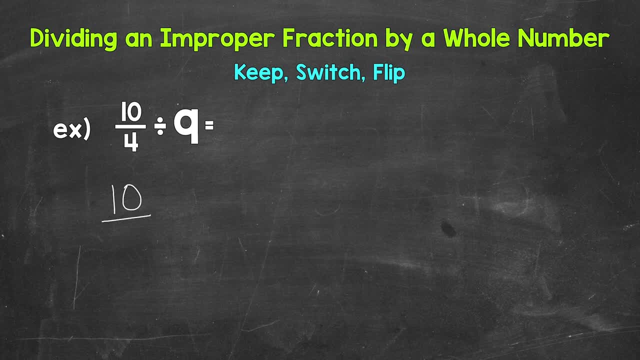 Let's keep 10, fourths, Switch to multiplication And then we need to flip that 9.. Well, we flip that 9 by writing it in fractional form. And remember, we can write any whole number in fractional form by putting it over 1.. 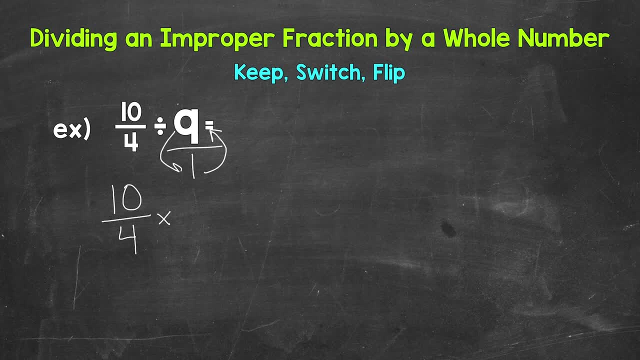 And now we can flip it So 1.. 1. Is the numerator And 9 is the denominator. So keep, switch, flip And then we can multiply straight across. now We will start with the numerators: 10 times 1 is 10.. 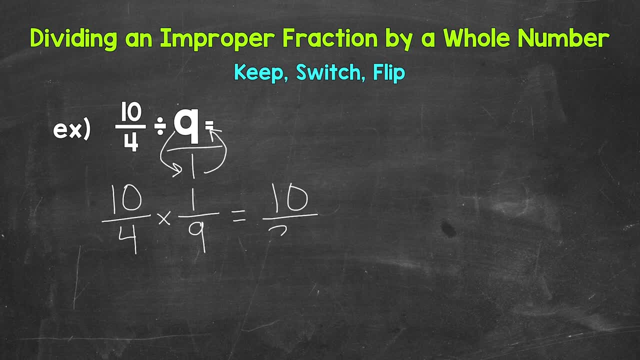 Now for the denominators: 4 times 9 is 36.. So we get 10 36ths or 10 over 36.. Which is our final answer. But we can simplify. We have a common factor other than 1 between 10 and 36.. 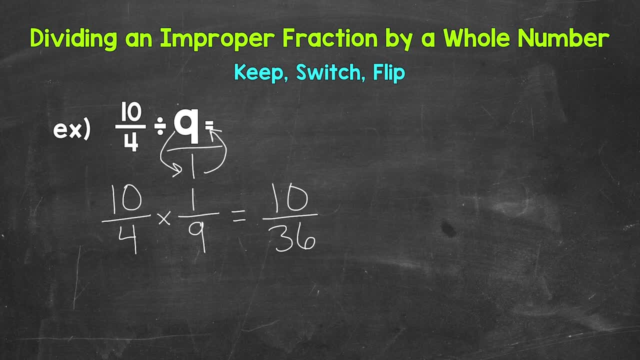 There is a greatest common factor of 2.. So let's divide 10 by 2 and 36 by 2 in order to simplify: 10 divided by 2 is 5.. 36 divided by 2 is 18.. The only common factor between 5 and 18 is 1.. 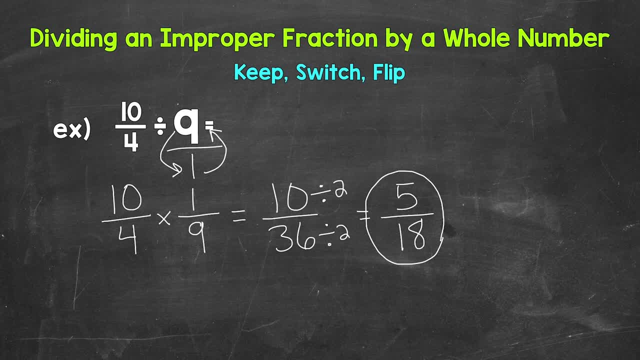 And 36 divided by 2 is 18.. So this is in simplest form. Final simplified answer: 5- eighteenths. So there's how to divide an improper fraction by a whole number. Let's move on to dividing a whole number by an improper fraction. 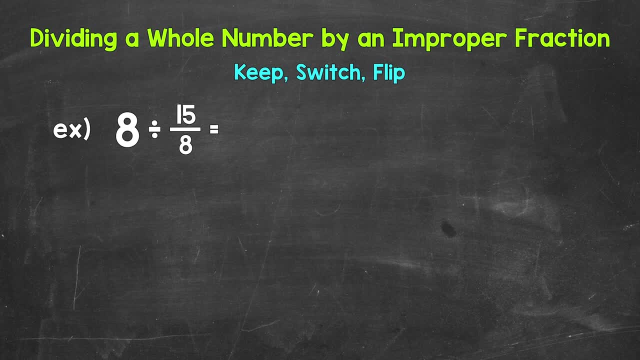 Now let's take a look at dividing a whole number by an improper fraction. Let's jump into our example where we have 8 divided by 15 eighths. So keep, switch flip, Let's keep 8.. Let's keep 8.. 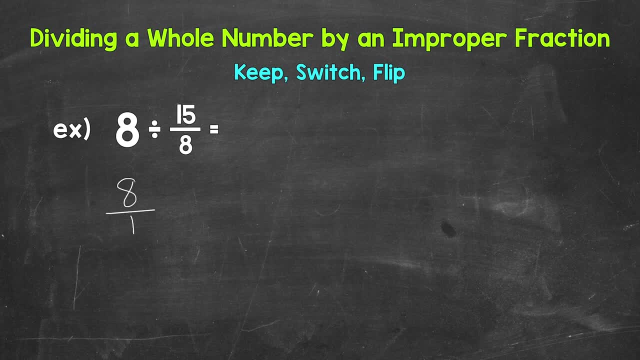 And I'm going to write it in fractional form. That way we have a numerator and a denominator. And remember, we can write any whole number in fractional form by putting it over 1.. So keep 8.. And again, we wrote it in fractional form. 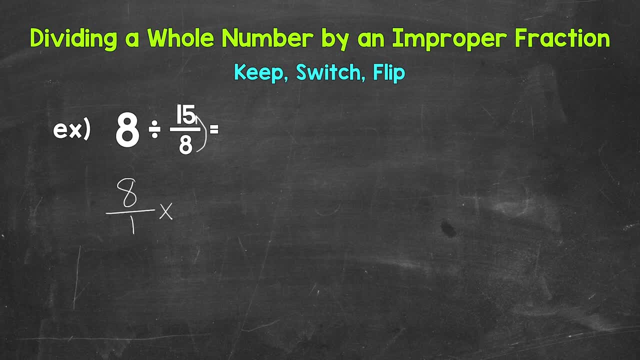 Switch to multiplication And then flip 15 eighths. So 8 is now the numerator And 15 is now the denominator. Now we can multiply straight across. Let's start with the numerators: 8 times 8 is 64.. 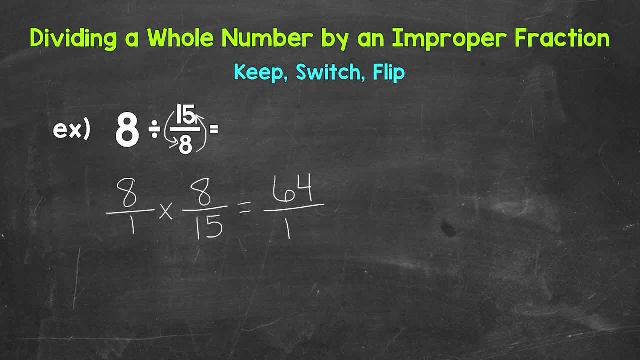 Now for the denominators: 1 times 15 is 15.. So we get 64 fifteenths, And that is our answer. But it's an improper fraction, So let's convert it to a mixed number by dividing the numerator. 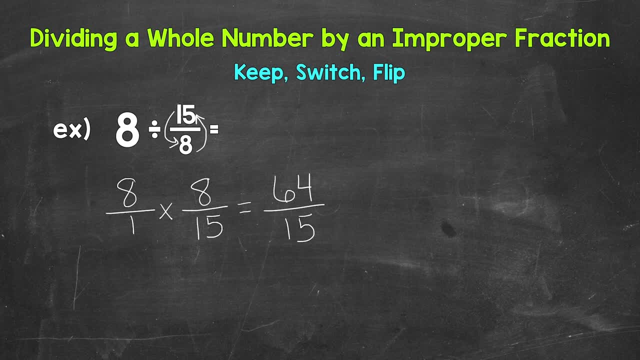 64 by the denominator 15.. So 64 divided by 15. How many whole groups of 15 in 64?? Well, 4. 4 whole groups. That gets us to 60. We don't hit 64 exactly. 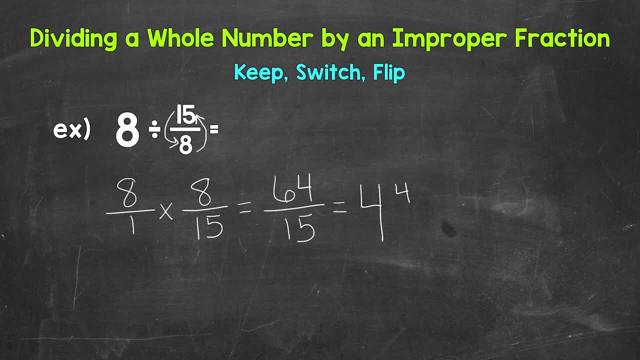 We have a remainder of 4.. That's the numerator of the fractional part of the mixed number, And then we keep the denominator of 15 the same. We can always look to see if we can simplify the fractional part of a mixed number. 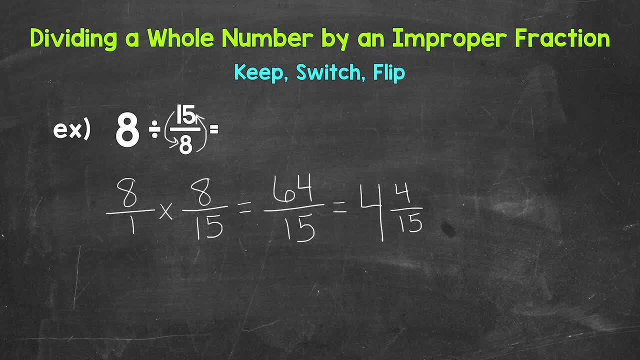 4- fifteenths is in simplest form. So final answer: 4 and 4- fifteenths. Now, just as a quick recap as far as how we went from that improper fraction, 64 fifteenths, to the mixed number of 4 and 4 fifteenths. 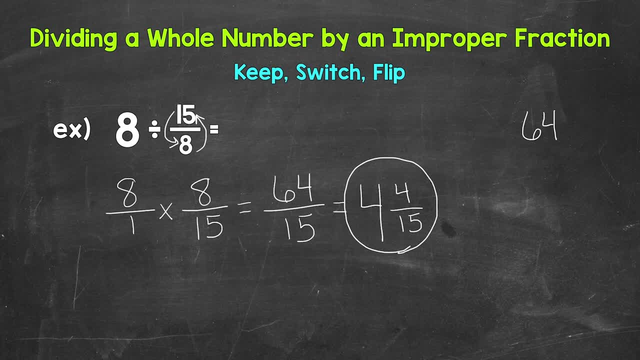 I'm going to write that out off to the side. so we did the numerator 64 divided by the denominator 15. so we have 64 divided by 15. how many whole groups of 15 in 64? well, 4, that's the whole number of. 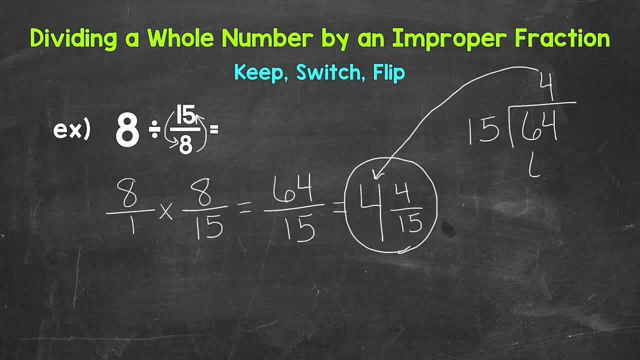 our mixed number. now we multiply 4 times: 15 is 60. subtract 64 minus 60 gives us 4. so we have 4 remainder 4. that remainder is the numerator of the fractional part of the mixed number. and then we keep the denominator of 15 the same. so there's how. 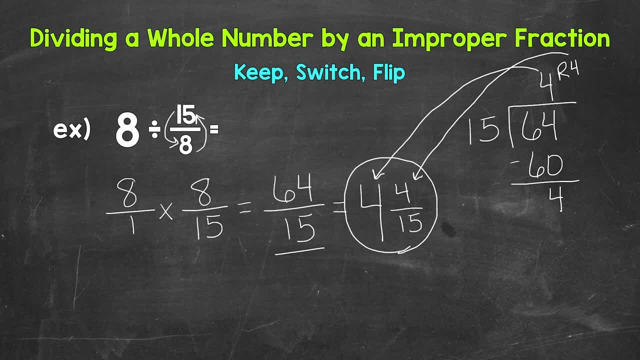 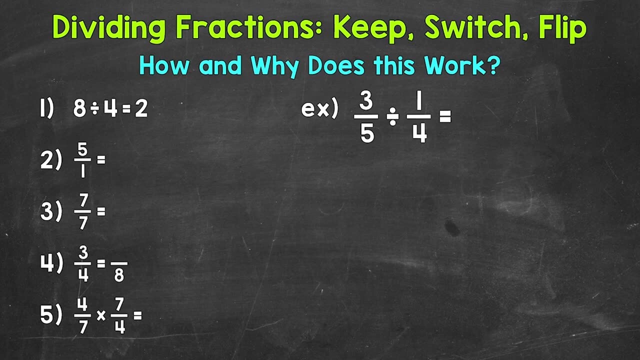 to divide a whole number by an improper fraction. let's move on to taking a look at why we use keep switch flip when we have division problems involving fractions. now we will take a look at why we use you keep switch flip when we have division problems involving fractions. You may also hear keep. 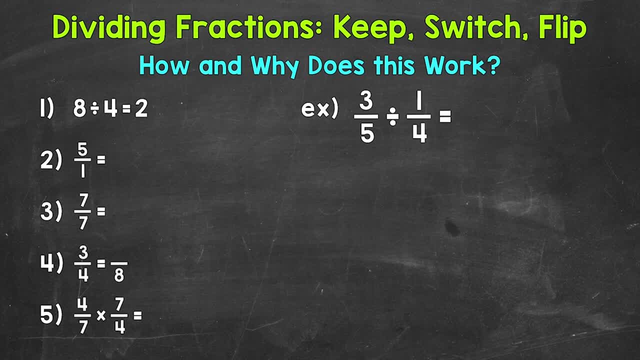 change, flip or multiply by the reciprocal. These all mean the same thing. Now, before we get into our dividing fractions example, we need to review and fully understand a few things about fractions. We'll start with fractions representing division. A division problem can be set up as a fraction, So 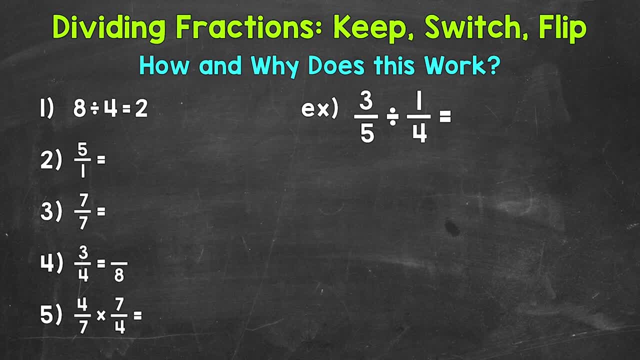 for number one, we have: 8 divided by 4 equals 2.. Now we can set that up as a fraction. We can set it up as 8 divided by 4 equals 2.. So again we need to know that fractions represent division. The second: 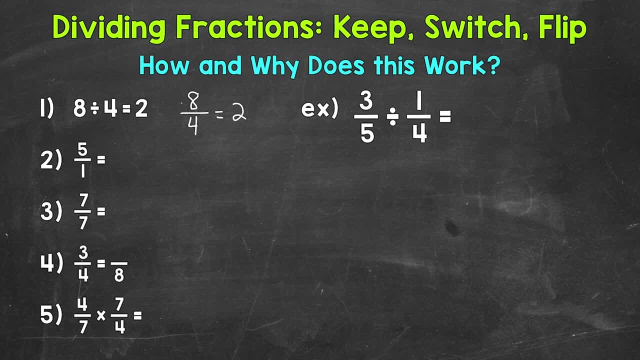 thing that we need to understand is that anything over 1, so a denominator of 1, equals itself. For example, 5 over 1 equals 5.. So again, anything over 1 equals itself. On to number three. here we have fractions that have the 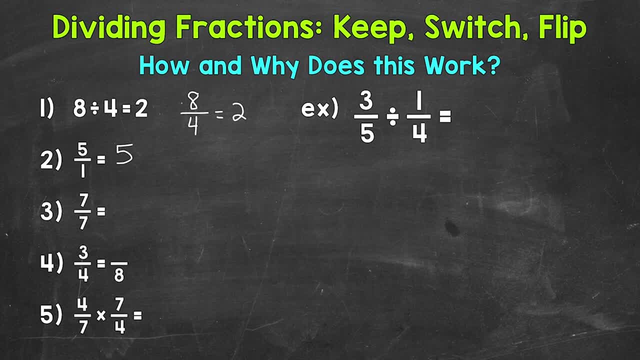 same numerator and denominator. For example, 7 over 7,, 7 sevenths. Anytime the numerator and denominator are the same, that fraction represents one whole. So 7 sevenths or 7 over 7, this equals 1. Again. 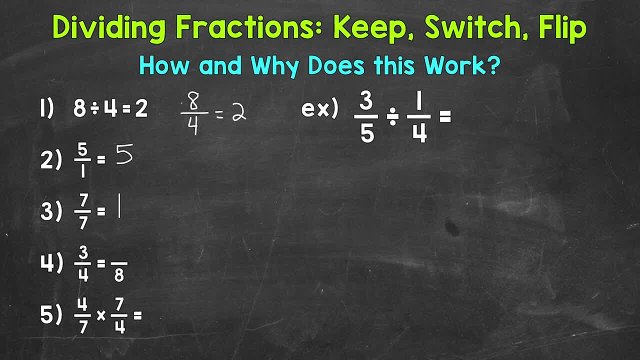 same denominator. same denominator equals 1.. The fourth thing that we need to understand: equivalent fractions. Now remember, in order to keep a fraction equivalent, whatever we do to the bottom, we must do to the top or vice versa, And we can use multiplication or division. This will 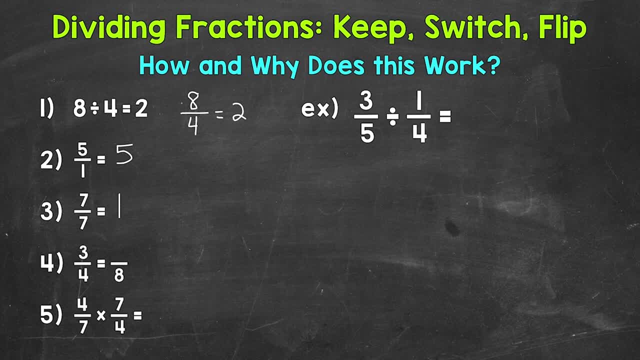 give us an equivalent fraction. For example, three-fourths equals how many eighths? Well, we know that 4 times 2, equals 8.. Now, whatever we do to the bottom, we must do to the top in order to keep this equivalent. 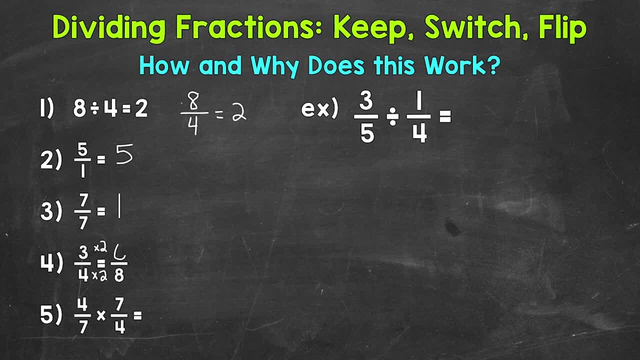 So 3 times 2, gives us 6.. So 3 fourths is equivalent to 6 eighths. Both of these fractions have the same value, So we need to understand equivalent fractions. Lastly, number 5: here we have: 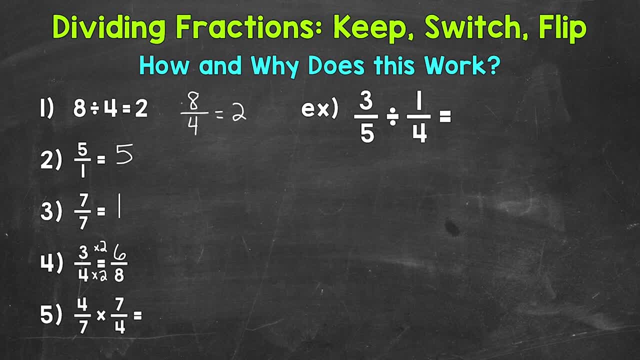 reciprocals, which is flipping a fraction. So the reciprocal of 4 sevenths is 7 fourths. So this is the reciprocal of 4 sevenths. Now I'm multiplying 4 sevenths by its reciprocal 7 fourths to show. 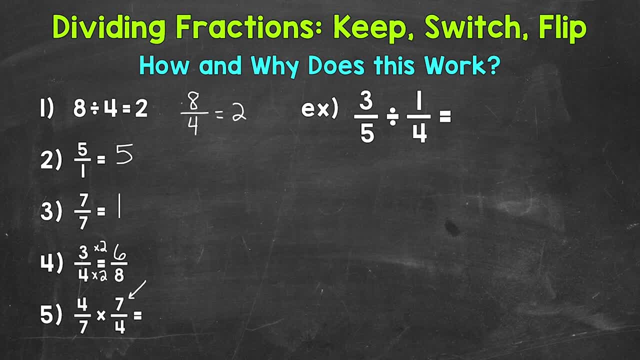 that we get 1 whenever we multiply a fraction by its reciprocal. So 4 sevenths times 7, fourths. well, multiply straight across: 4 times 7 is 28.. Now let's multiply the denominators, the bottom numbers, 7 times 4 is 28.. So we end up with 28- 28ths. And we know that if we have 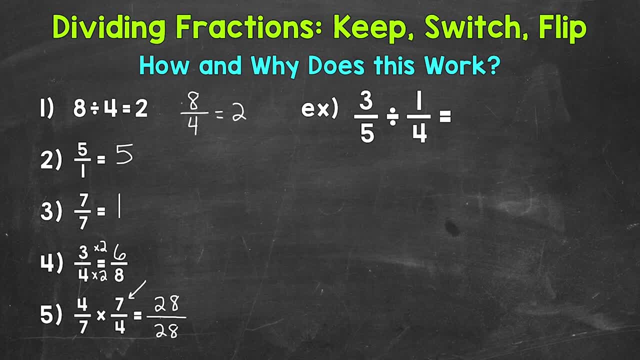 the same number on top, the numerator, as we do the bottom, the denominator. this is going to equal 1 whole or 1.. So reciprocals are the last thing that we need to understand. And again, a reciprocal: We flip the fraction, The numerator becomes the denominator and the denominator becomes. 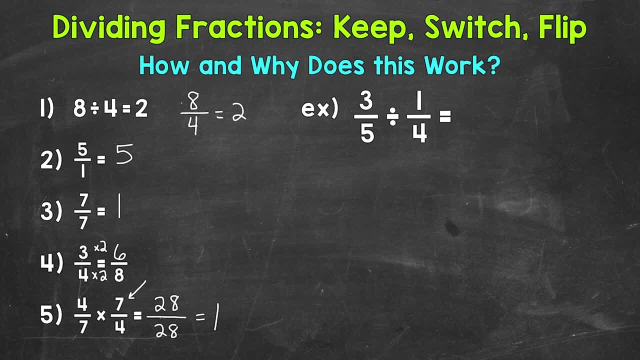 the numerator And when we multiply a fraction by its reciprocal, we get 1.. Now we are ready to see why we keep switch, flip- Or maybe you refer to it as keep change, flip, or multiply by the reciprocal. Remember, all of those things mean the same thing. Let's use 3 fifths divided by 1. fourth, 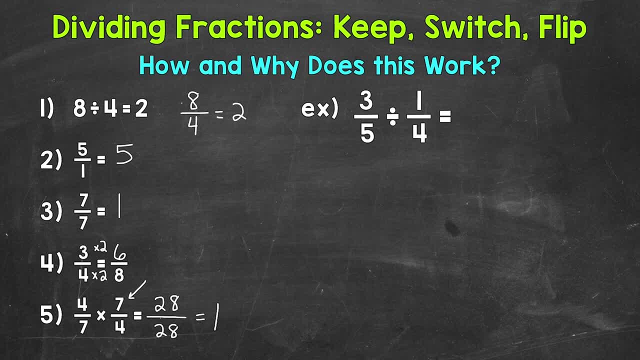 for our example, 3.2 divided by 1 is definitely the best move. We know that we can set up a division problem as a fraction. Fractions represent division. So let's set up 3 fifths divided by 1 fourth. as a fraction, We geth 3 fifths over 1 fourth. 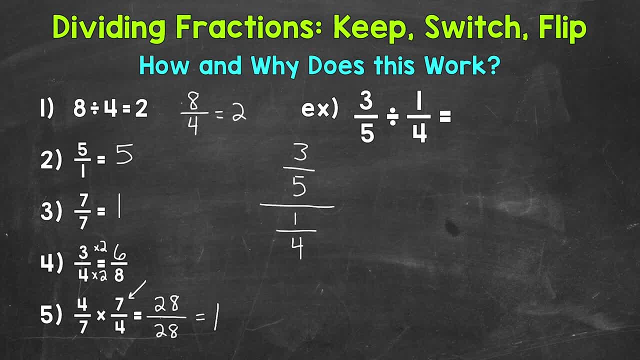 This gives us a fraction over a fraction. So two fractions are making up 1, fourth up one fraction. This is called a complex fraction. A complex fraction is a fraction where the numerator, denominator or both are a fraction. Now, once we have our complex fraction, 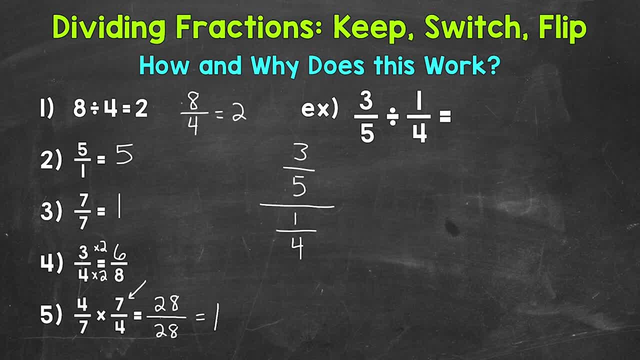 we want to get our denominator to equal one. We know that anything over one equals itself, and that is going to make this much more manageable. Well, how do we get our denominator to equal one? We need to multiply it by its reciprocal Flip, the fraction. So let's multiply. 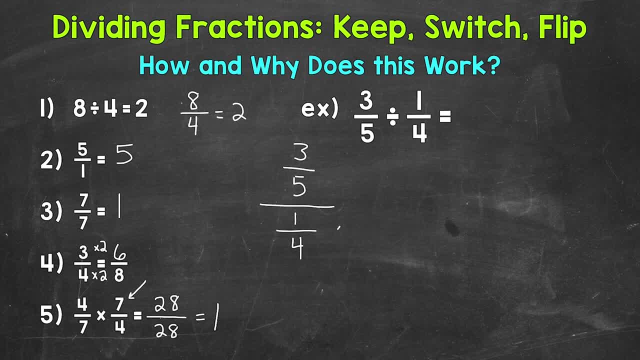 one-fourth by four over one. And again we are doing this, so we get that denominator to equal one, because we know that anything over one equals itself. Now, since we are multiplying our denominator to equal one, we need to multiply it by its reciprocal. So let's do that. 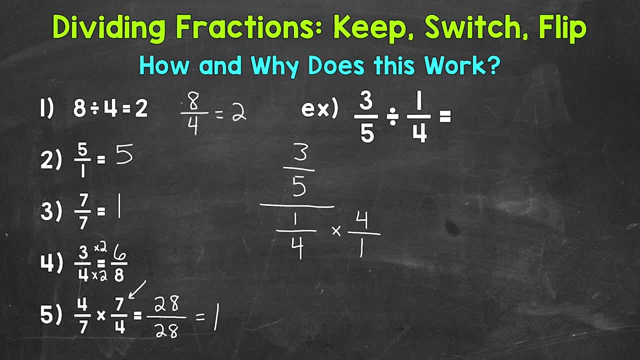 So let's multiply our denominator by four over one. Remember, in order to keep a fraction equivalent, whatever we do to the bottom, we must do to the top, or vice versa. This keeps everything equivalent. The value doesn't change. So we need to multiply our numerator by four over. 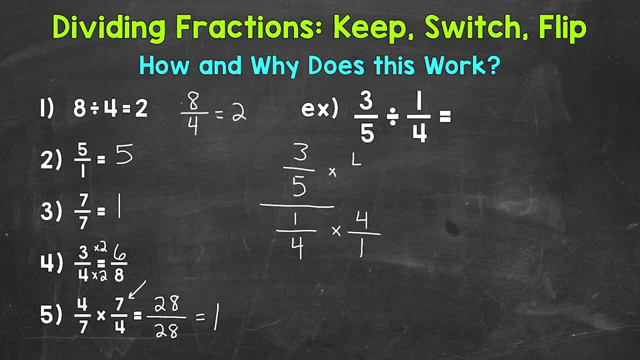 one as well. So this is going to give us: well, one times four is four, four times one is four. Remember, when we multiply fractions, we multiply straight across. So again, one times four is four, and then four times one is four. Let's do our numerator So. 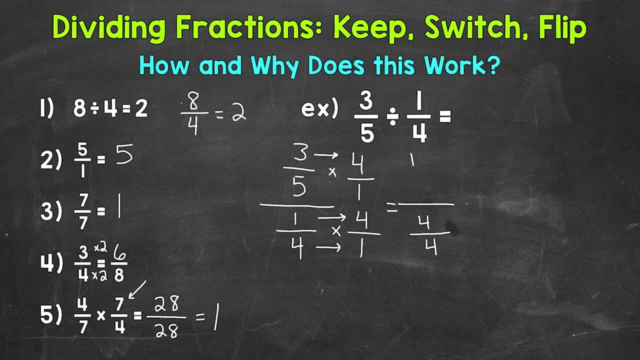 three times four, right here- is going to give us twelve, and then five times one is going to give us five. So we have twelve-fifths over four-fourths. Now we know that when we multiply fractions, we have the same numerator and denominator: The fraction equals one. So let's rewrite this: 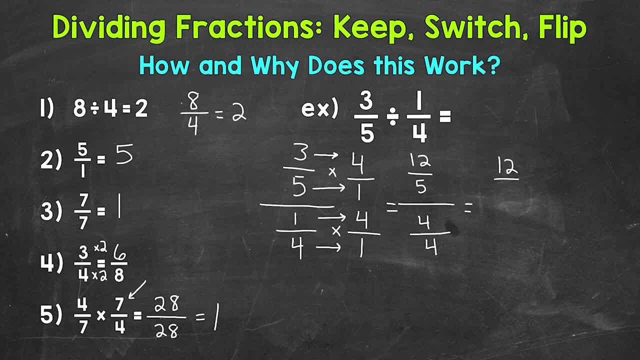 as twelve-fifths over one. This is our new complex fraction. It's equivalent to what we started with, but now we have a denominator of one and we know that anything over one just equals itself. So our answer is twelve-fifths. Now, twelve-fifths is an improper fraction, so we want to change this to a 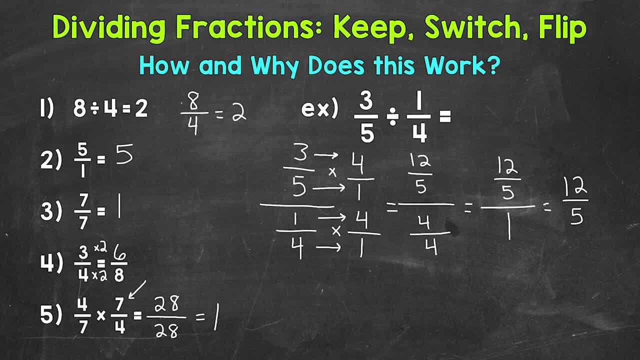 mixed number. We do that by dividing our numerator by the denominator. So twelve divided by five, How many whole groups of five can we pull out of twelve? Well, two, Now, that doesn't hit twelve exactly. We have a remainder of two and we keep that. So we have a remainder of two and we keep. 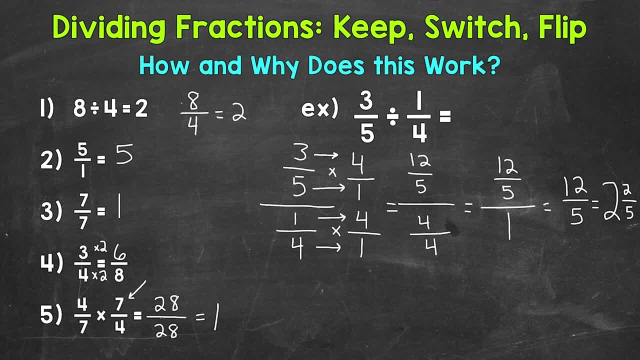 our denominator of five. the same Now two and two-fifths. our fractional part is in simplest form. so we are done. Two and two-fifths is our answer for three-fifths divided by one-fourth. So you can see that that was a fairly long process. That's the long way of dividing fractions. It does work. 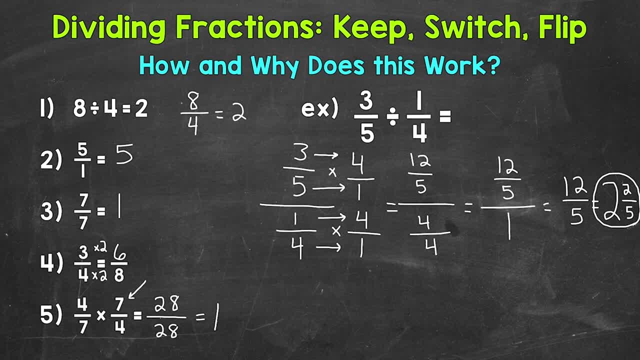 but we can use keep switch flip to be more efficient. Let's try keep switch flip as well and see how everything compares. So I'm going to rewrite the problem at the bottom of the screen here. So we have three-fifths divided by one-fourth. So let's keep switch flip. So keep our first fraction three-fifths, switch to multiplication and then flip our second fraction. 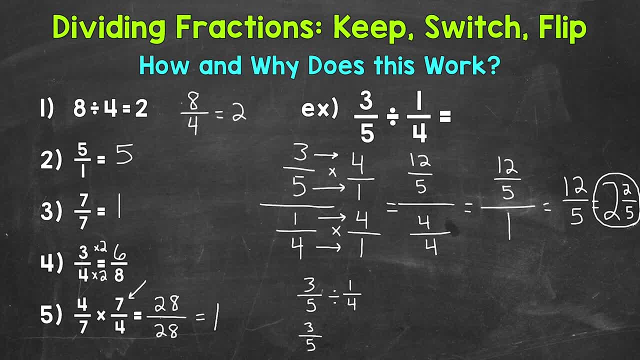 So keep our first fraction three-fifths, switch to multiplication and then flip our second fraction. we get 4 over 1 and then we multiply straight across. we get 12 fifths- the same answer we got when we used the long way, and we convert this to a mixed number, which is 2 and 2 fifths. so you can.